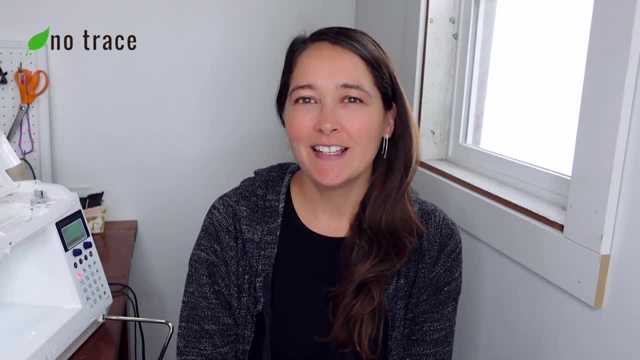 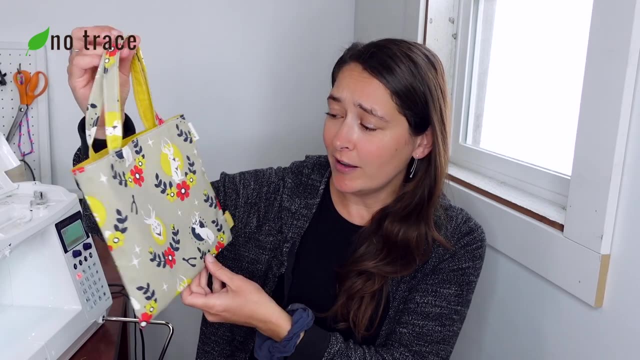 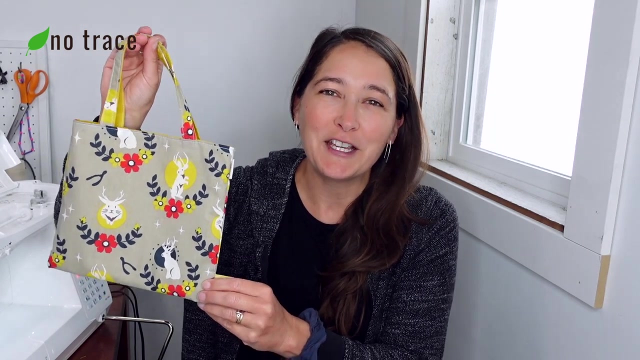 Hey, there, it's Liz from No Trace. Welcome back to my channel. In this video I'm going to show you how to make this adorable mini tote bag. A couple of years ago, at a holiday craft fair, I got each of my daughters a bag just like this from another maker here in town And they just loved the bag. 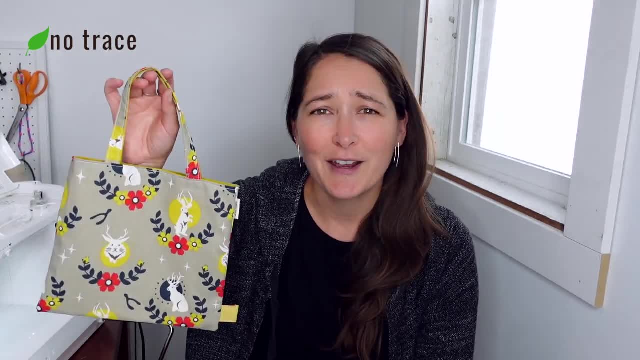 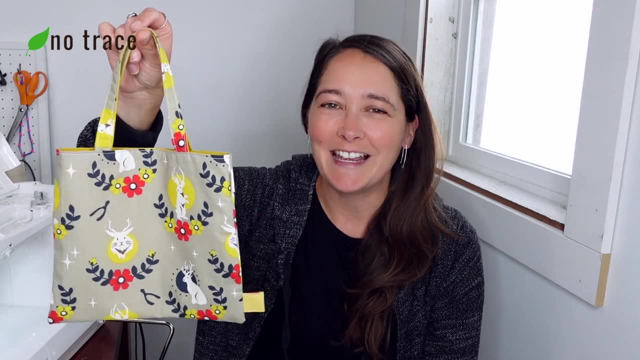 They still use the bag. They put little hair supplies in it or art supplies in it, And I knew I had to figure out how to make it and make one for you. So that's what we're going to do today. So let's go. 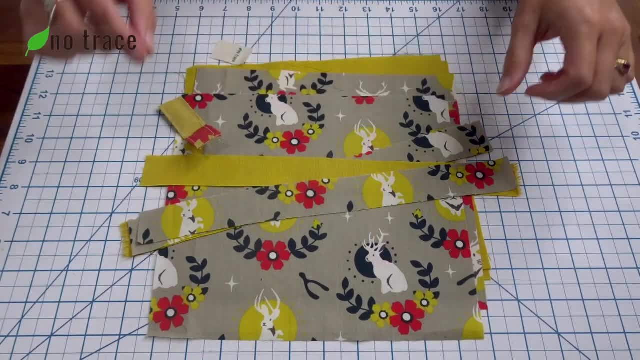 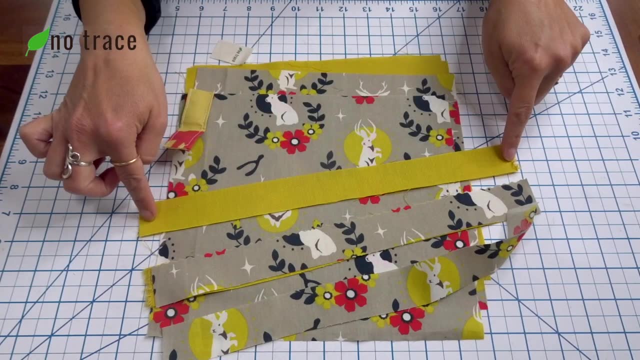 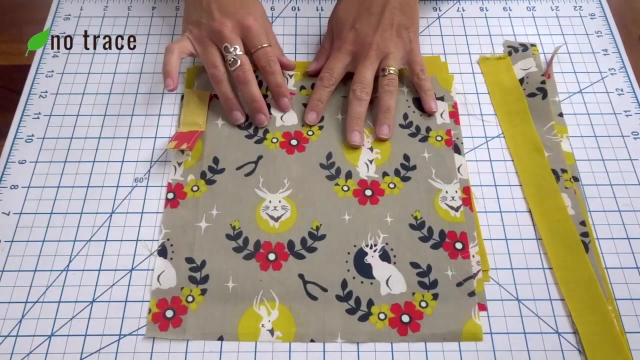 In order to make your mini tote bag, you're going to need four pieces of material to make the straps. These are all 12 and a half inches long And one and a half inch tall. Then you're also going to need four pieces of fabric to make. 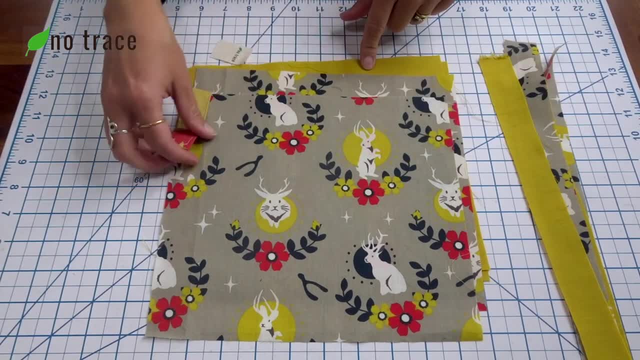 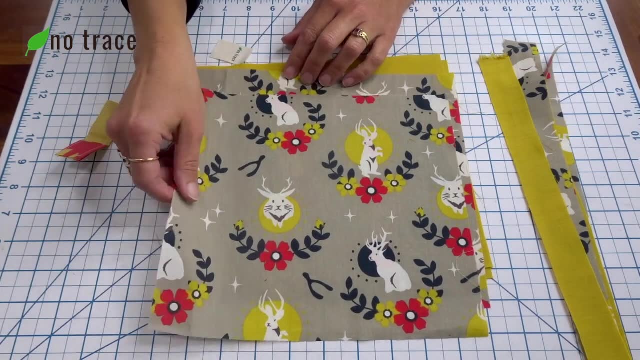 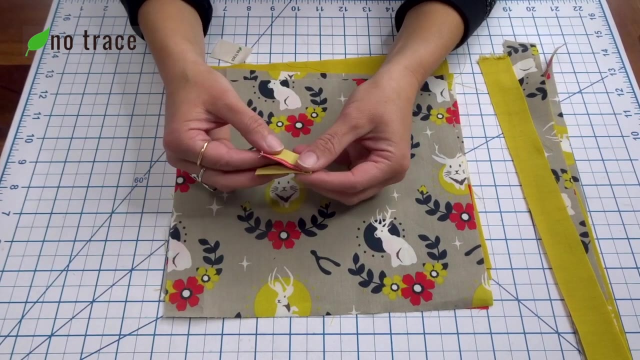 the outer layer and the inner layer of your pouch, And my pieces are all 10 inches wide and nine inches tall, So I have two for my outer and two for my inner. Then you can also, if you want to add a little bit of bling to your bag, have a little piece of three inch ribbon. 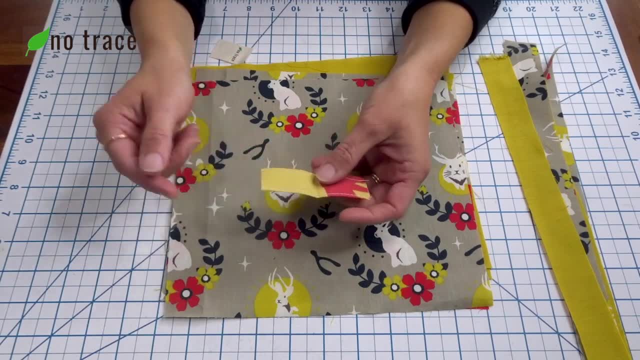 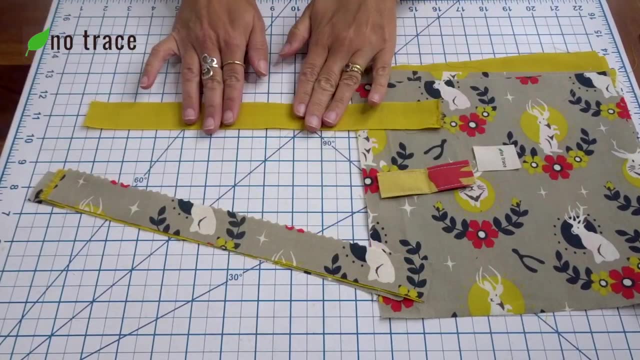 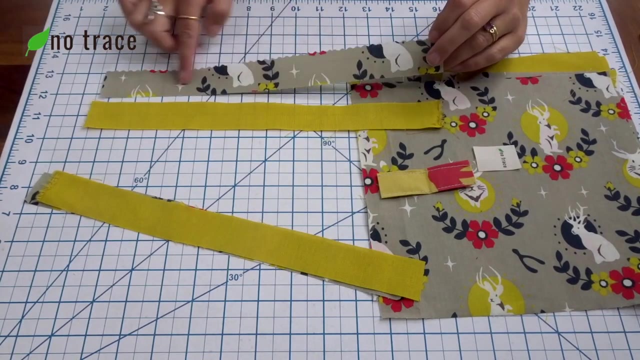 or a three inch piece of strap that coordinates with your other layers. The first step is to assemble your straps, So what you want to do is put two pieces of strap material with the right sides together. So I'm using one of my outer, a scrap from the outer fabric and a 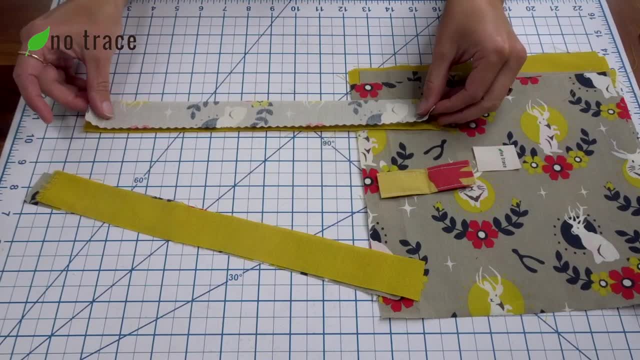 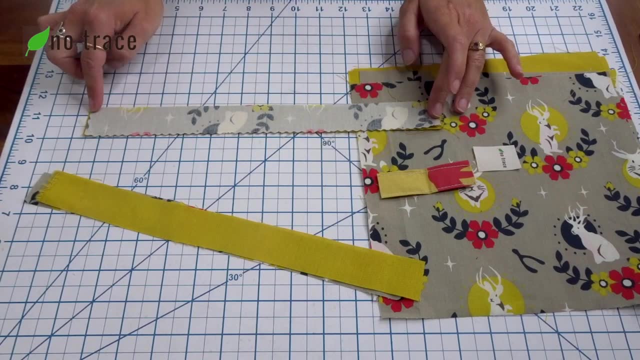 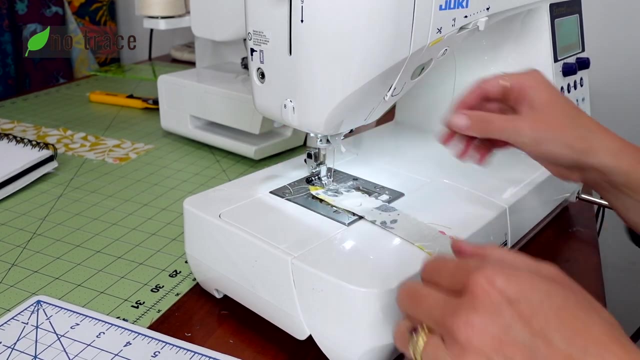 scrap from the inner fabric right sides together And we're going to stitch along the long edges with a quarter inch seam allowance. So over my machine I'm going to lift my presser foot and just sew pretty close to the edge with about a one quarter inch seam allowance all the way down. 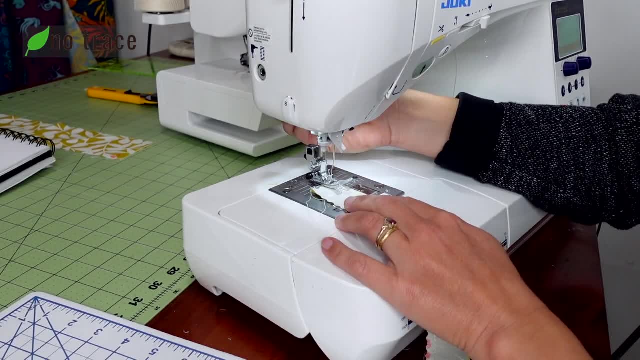 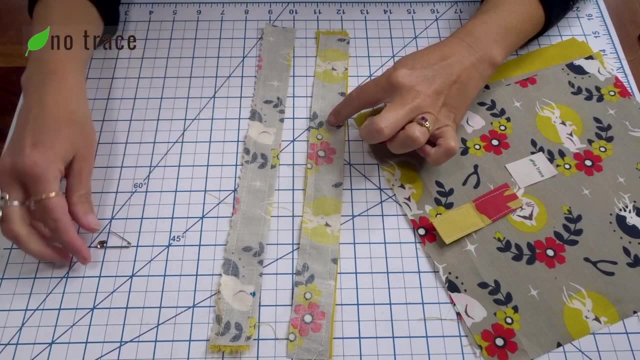 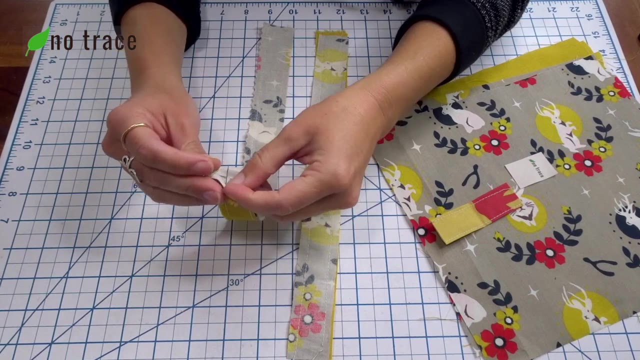 And once you've stitched one side, just go ahead and repeat on the other side. Once you've stitched the strap pieces together, you're going to want to take a safety pin and clip it to the other side, And then you're going to clip it to one end of your strap. 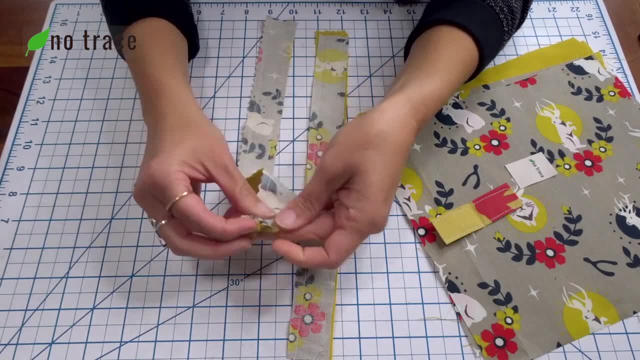 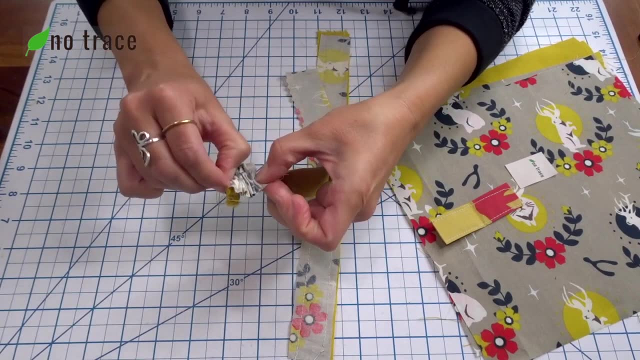 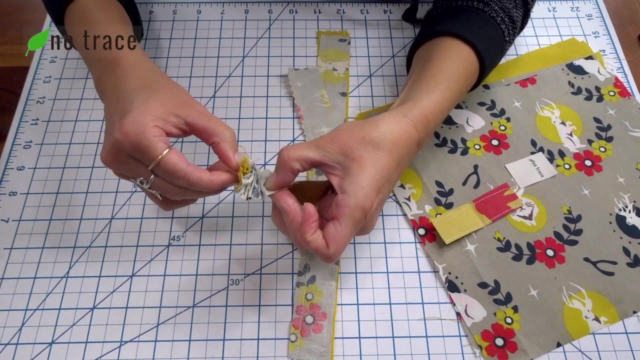 And then you're going to thread it all the way through to turn your strap right side out. Now, the larger the safety pin, the faster this will go, And if you sew a lot, you might want to get a tube turner, which makes this even faster. So I'll show you how to use that as well. 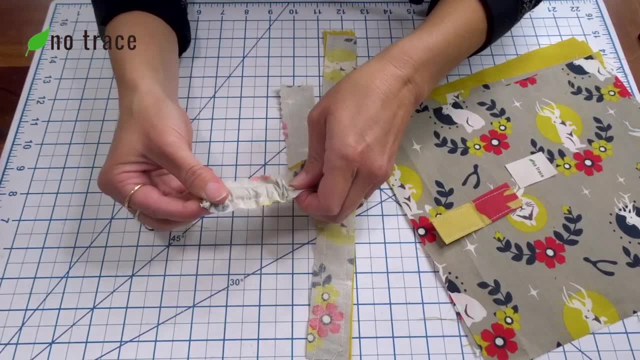 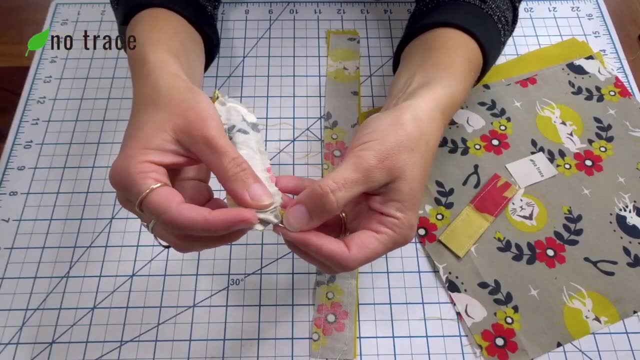 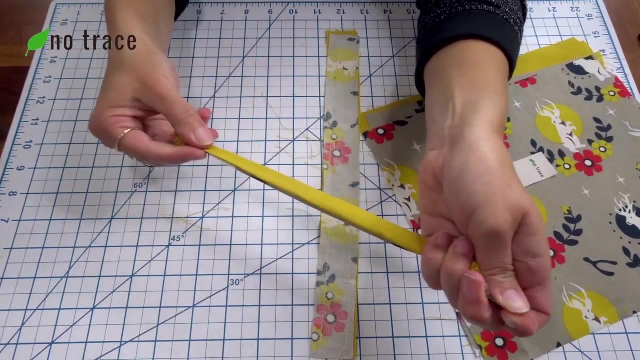 Just push it all the way through and then gently pull the fabric off the back end as the safety pin moves forward. And once the safety pin makes it to the other opening, just gently turn your tube right side out all the way And then take your pin off. 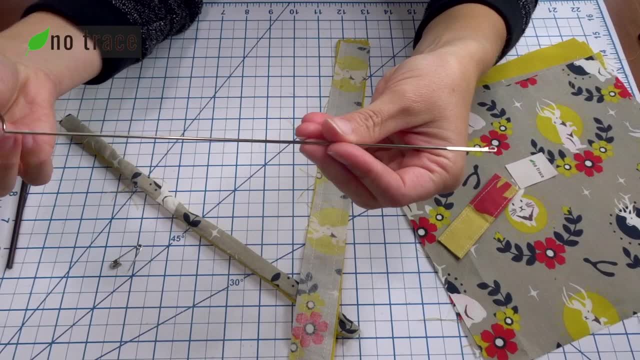 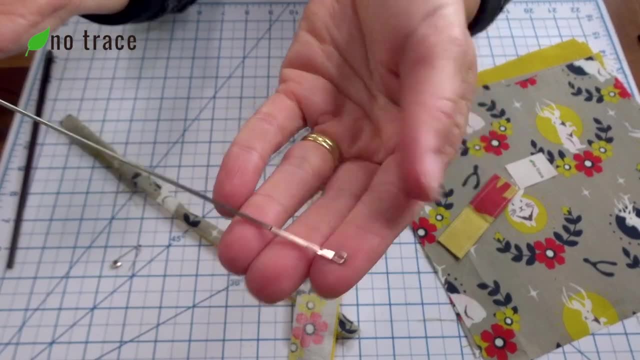 Another way to do this is with a tube turner. So that's this tool that has a little bit of a twist. It has a little ring at one end and it has a little bitty hook at the other end, So you want to get your tool inside the strap. 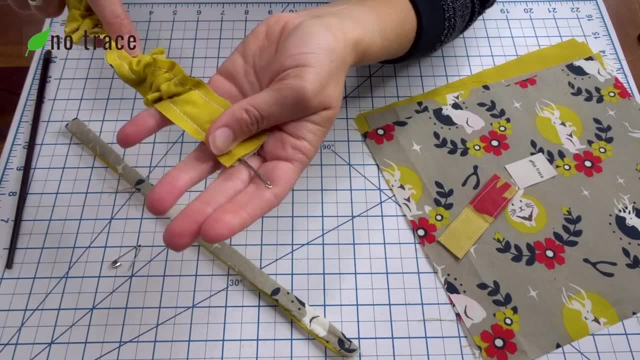 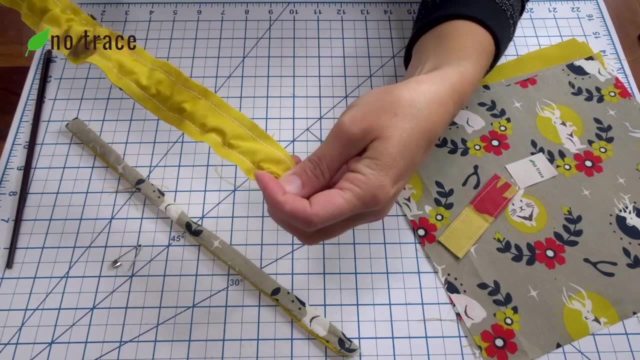 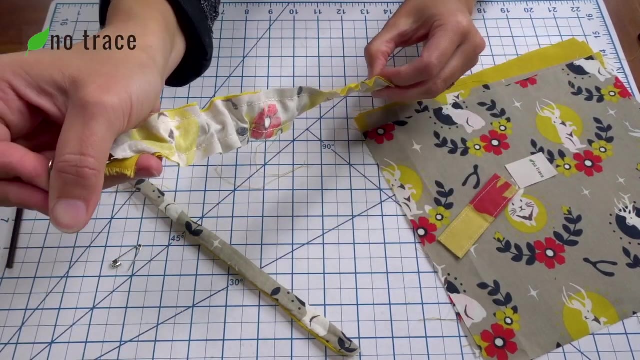 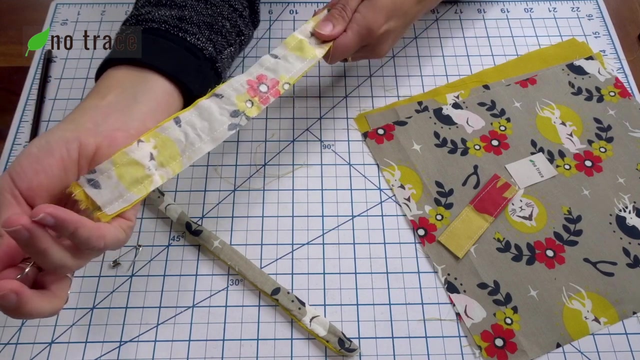 Push that hook to the opening of the strap And then you want to hook the little hook onto some fabric. Just get a pinch of fabric and then just gently tug on the tool on the ring end of the strap So that the fabric turns right side out. And you want to sometimes this little hook. 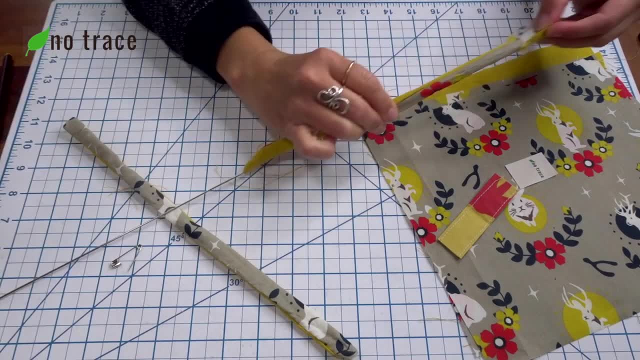 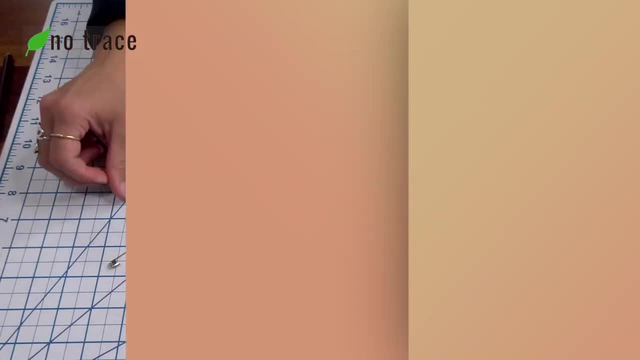 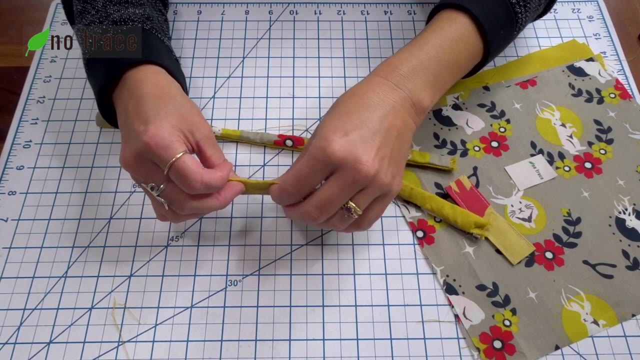 will hook on other fabric as you go, So just be gentle with it. and your tube is right side out. Next you'll want to make sure that the ends are all turned out nicely, And then you can kind of roll the seam in your fingers to try to make your strap. 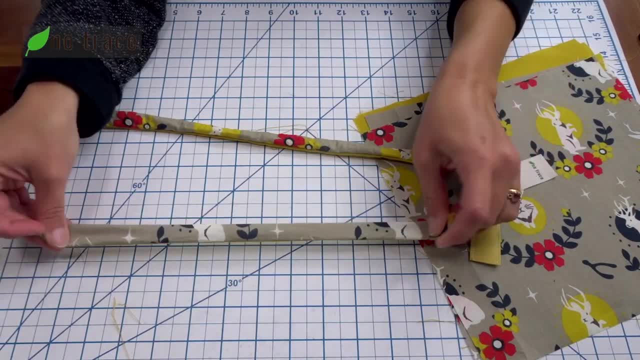 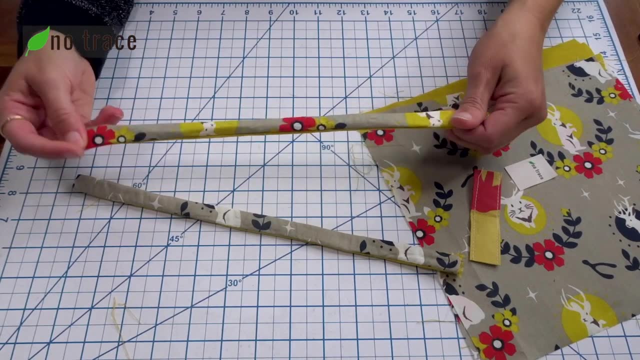 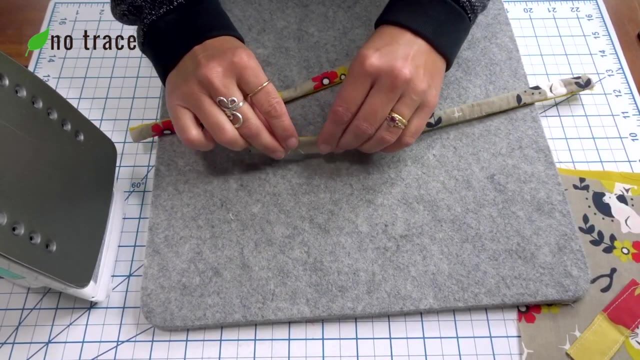 widen a little bit. So just feel that seam and make sure that the fabric isn't too bunched up along the seams, And then we're going to take this to the iron and really flatten these out. So again, just make sure that the strap is laying as flat as possible And then just press it. 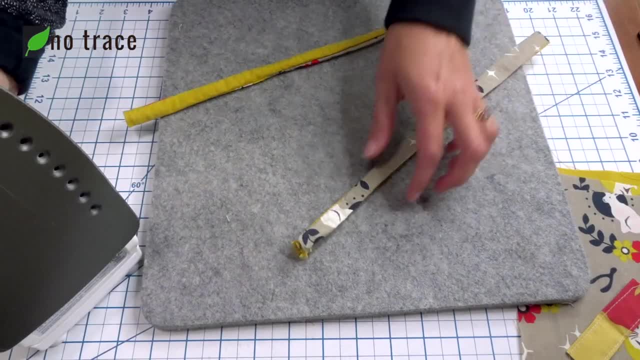 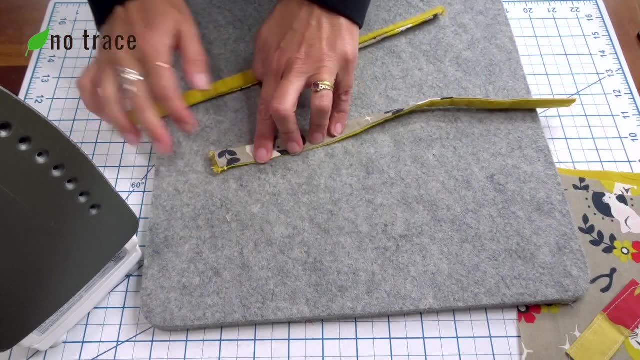 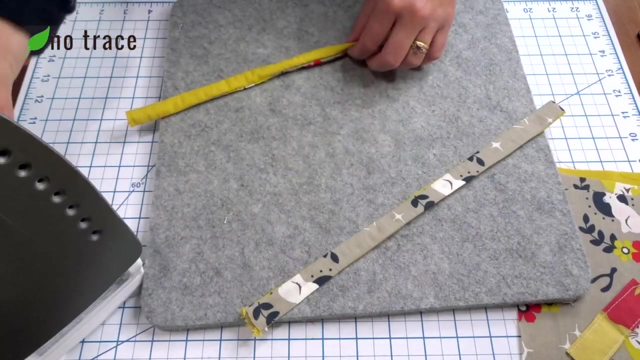 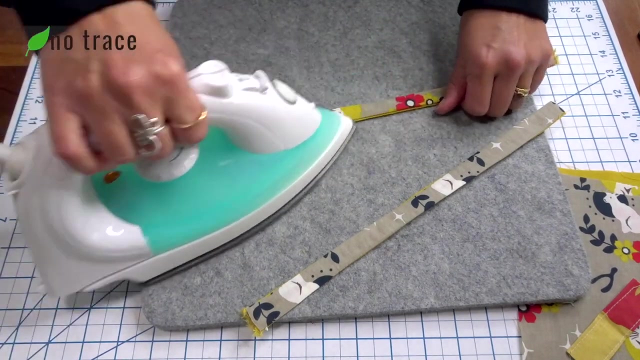 at the iron, Flip it and get the other side Again. make sure that you can kind of roll those seams out So that they lay nice and flat And then, with the iron, press on them And repeat that for the other strap. Once you're finished pressing each of the little straps, we're going to go. 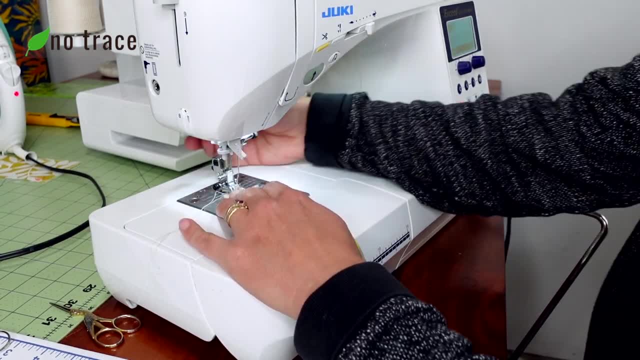 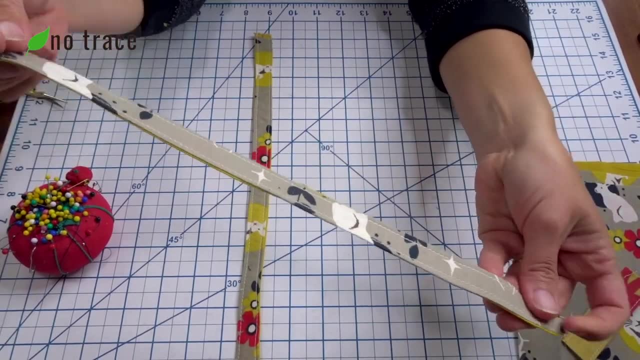 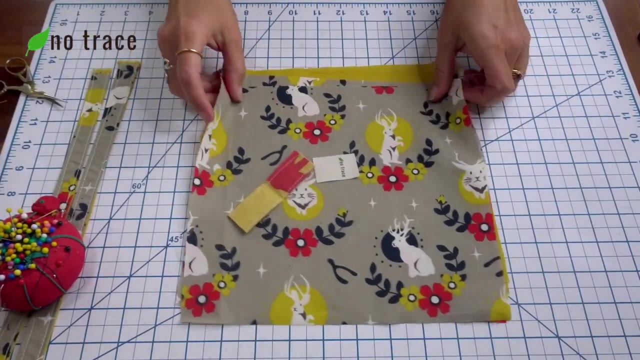 ahead and do a top stitch on both sides with about an eighth of an inch seam allowance. After you're done top stitching both sides of each of your straps, you can go ahead and set the straps aside for now, And what we're going to do next is assemble our panels of the bag. 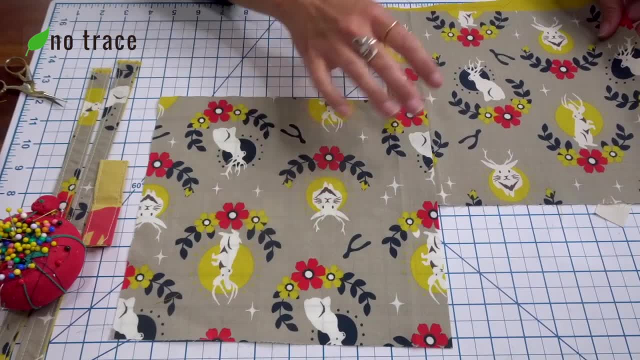 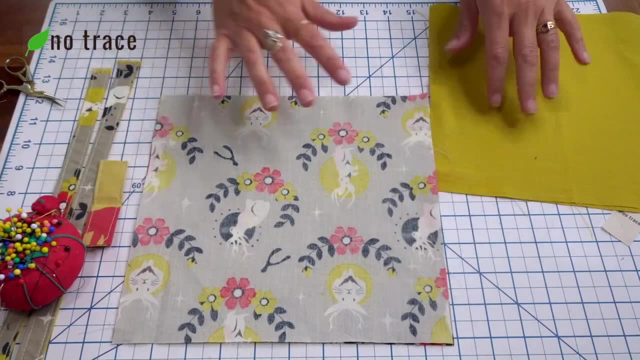 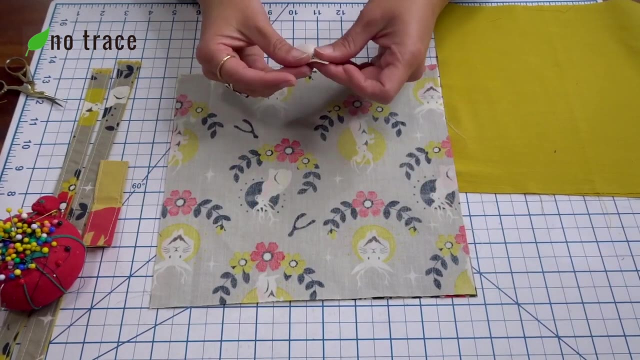 So let's start with the outer layers. We're going to put them with the right sides together And we're going to be stitching around all three sides, leaving the top opening, And I'm going to add a little tag that says no trace over on one side. 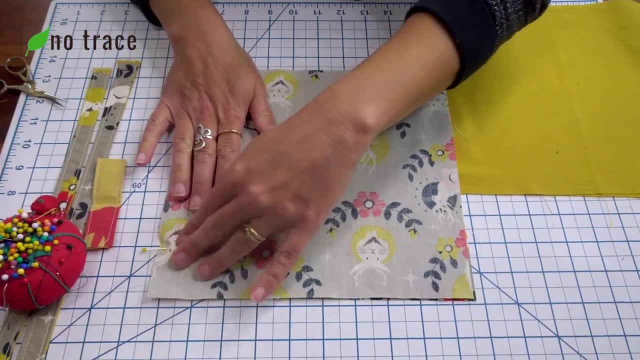 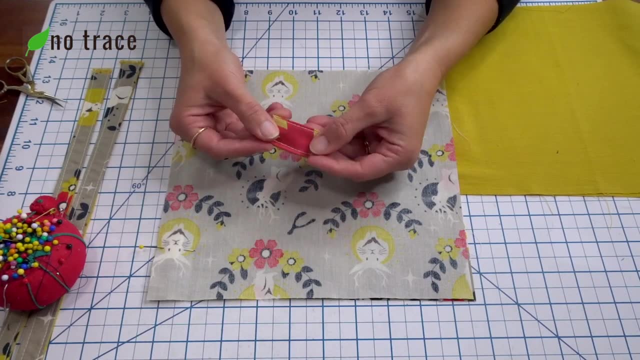 And then I'm also going to add this little ribbon. It just gives a little bit of personality to the bag And it's what I saw on the bag that I bought my kids, that I thought was cute. So we're just going to add a little loop just for fun. 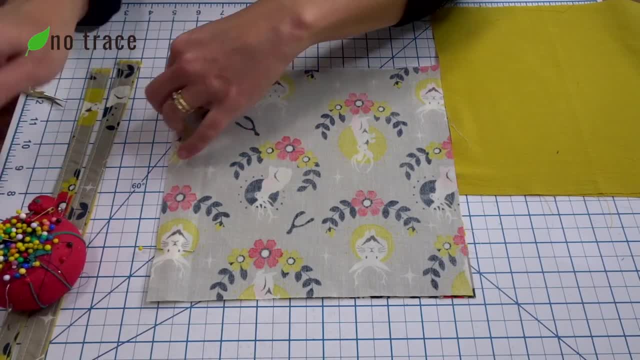 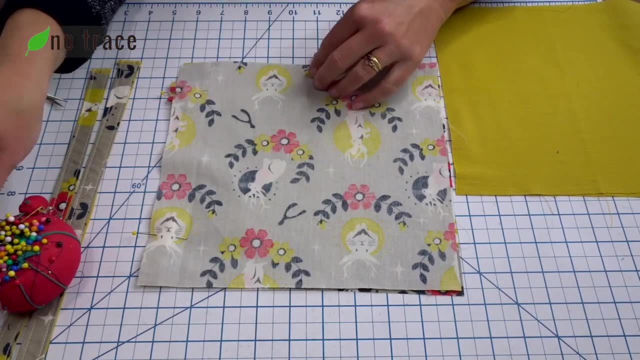 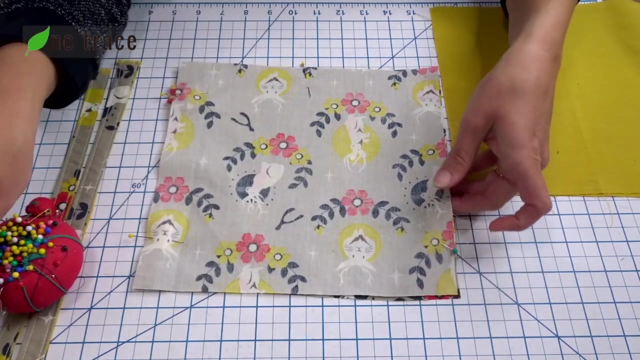 And we want it to stick out about a quarter of an inch And then go ahead and pin that, And then we're going to add a couple more pins. I don't need a ton of pins because I sew so much, But when you're starting you probably want to use. 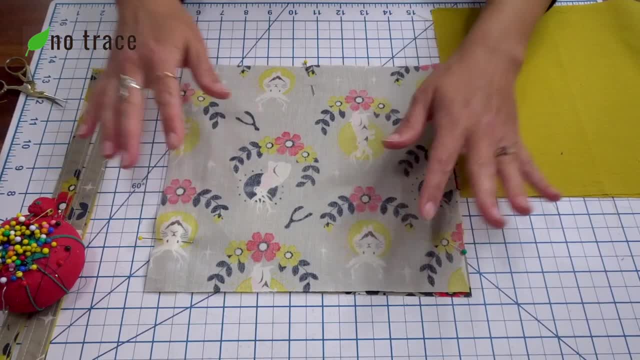 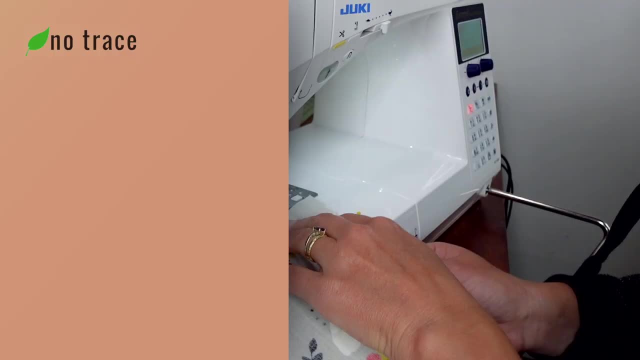 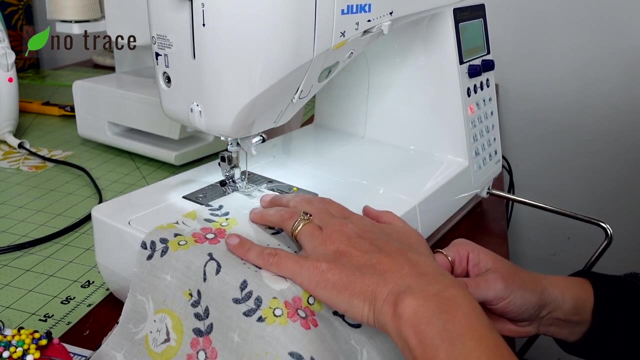 more pins And then we'll go ahead and take it to the machine and stitch all the way around with a half inch seam allowance, All right back at the machine- Half inch seam allowance, And we want to do a back stitch at the beginning, So go forward a few. 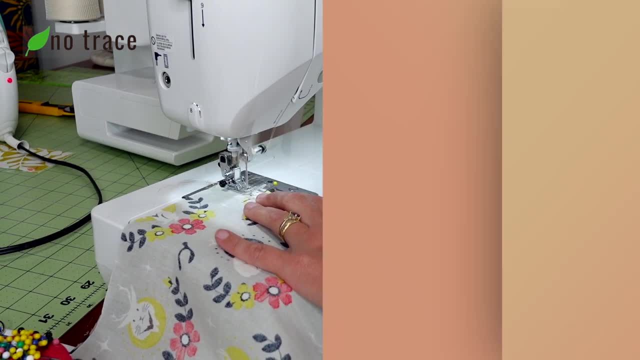 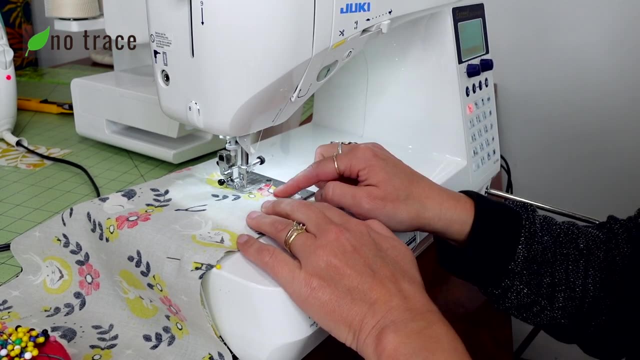 backward a few and then just straight down As we get near the strap. we're going to go over it a couple of times just in case you, the little one in your life, wants to tug on the strap so it really stays put- And then reverse. 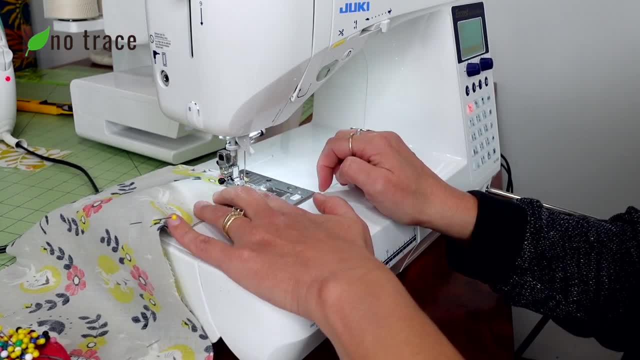 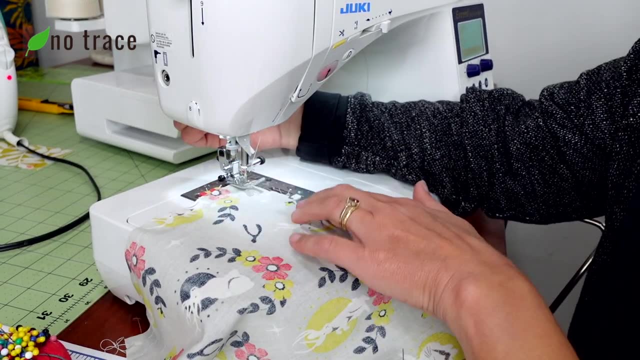 And All the way to the corner. When you get to your corner, when you're about a half inch away from your corner, go ahead and lift your presser foot, Keep your needle down and turn the bag And then continue down the next side. 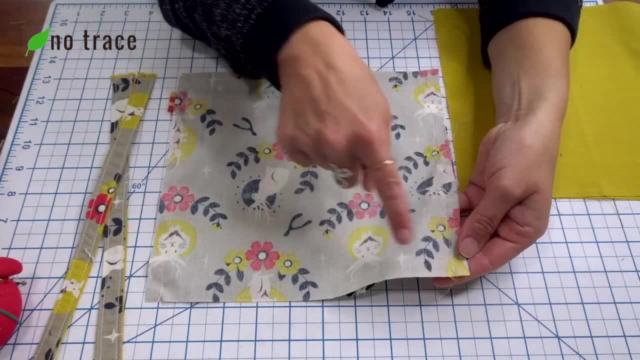 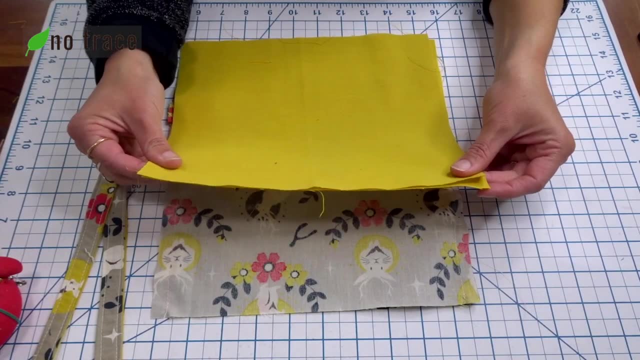 So I've stitched these three sides and I also did a little back stitch where I started and where I stopped. So now I'm going to do the same thing with my liner fabric, So I want to line it up with the right sides together. So this is where I'm going to start and where I stop, So I'm going to. 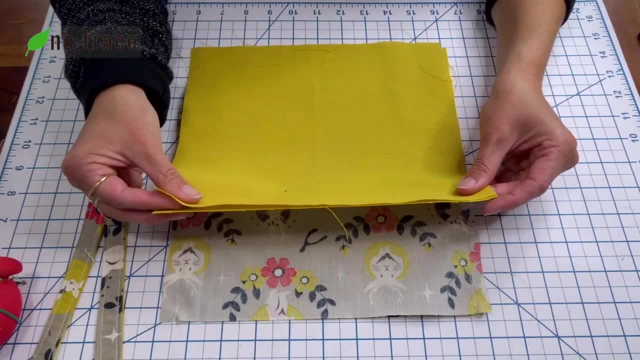 just stitch the two sides together so that it's all lined up nicely, And then I'm just going to go over the top of my edge right here. So if you want to stitch this side together, you can do that if you have a printed hemline. so if this is a solid, there is no right or wrong. 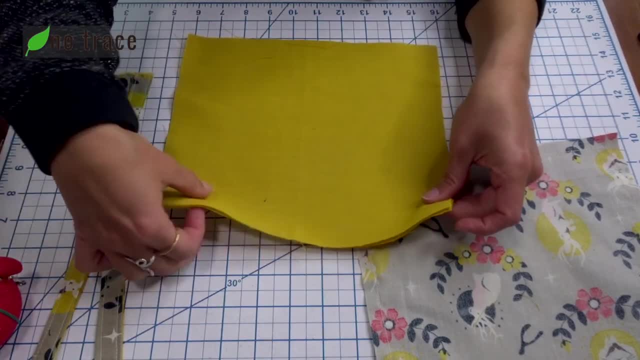 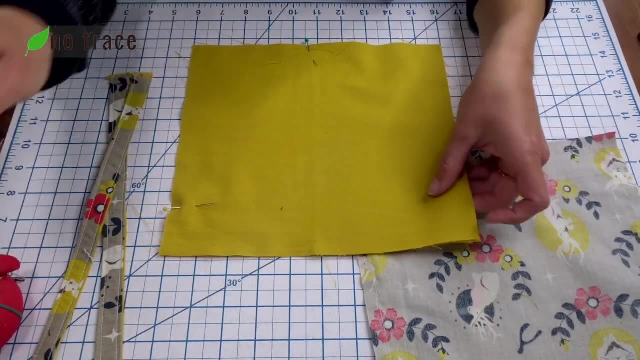 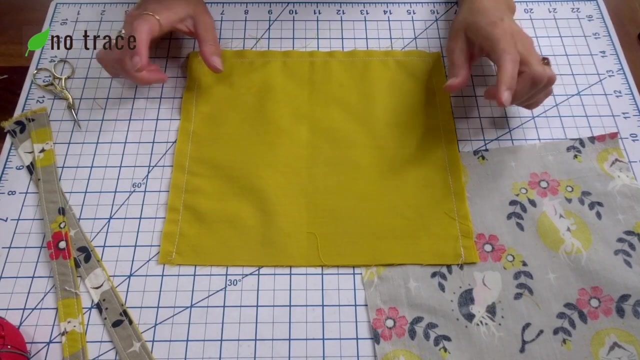 But if you have a print, you want right sides together, make sure all your edges are lined up nicely And then put some pins to keep things together. I'm just gonna do a few pins like this And then again I'm just gonna stitch these three sides. 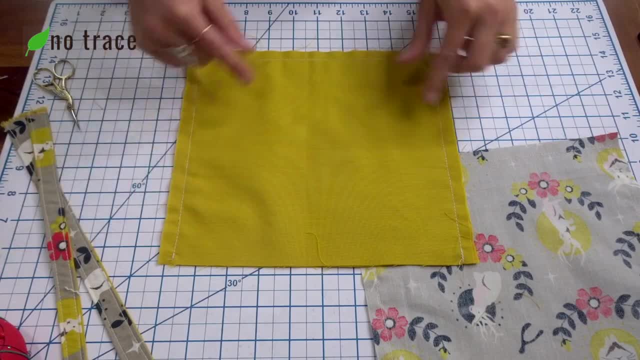 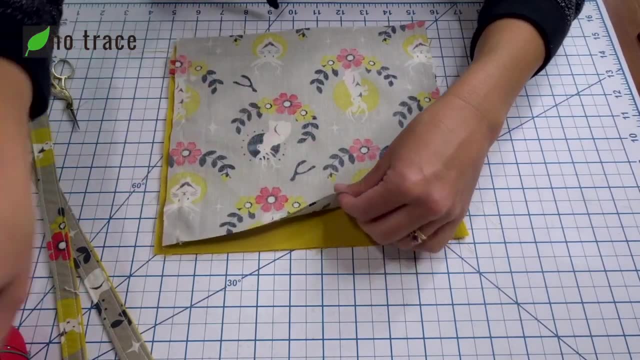 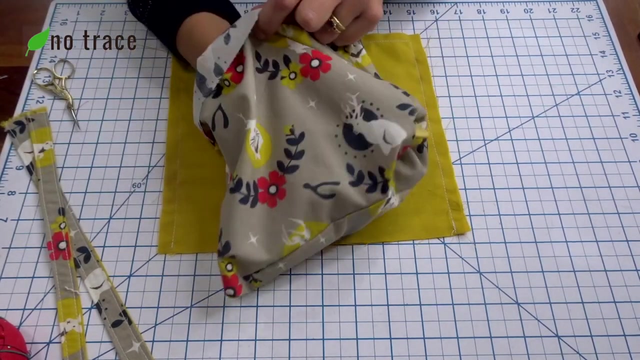 and our outer pieces are done, our straps are done. we're ready to assemble the bag, And the way we're gonna do that is we're gonna turn our outer pieces right sides out, just like that. Make sure those corners are pushed out. 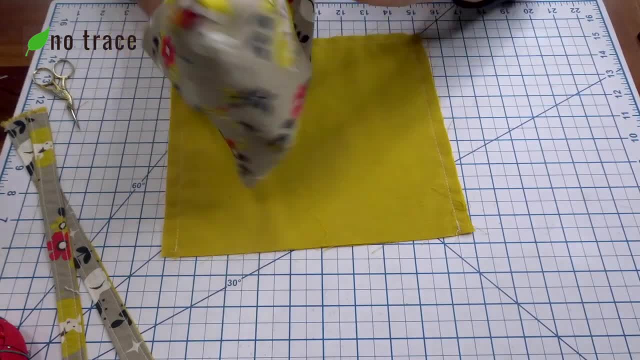 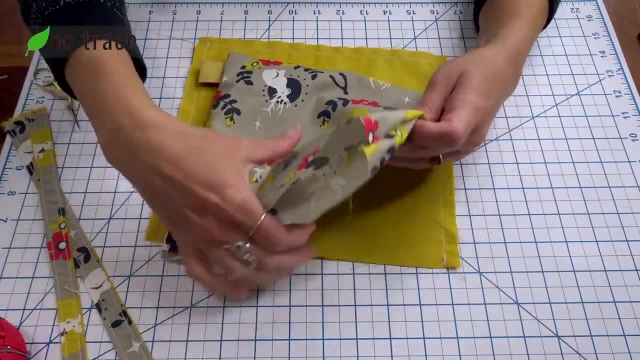 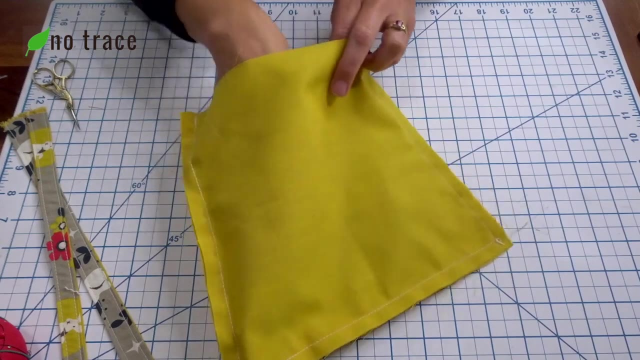 So I have a little chopstick, I'm just gonna get my corners pushed out, nicely, Okay, and now I'm gonna insert the outer fabric inside the liner fabric. The liner fabric is still turned wrong side out, Okay, so just get that inside. 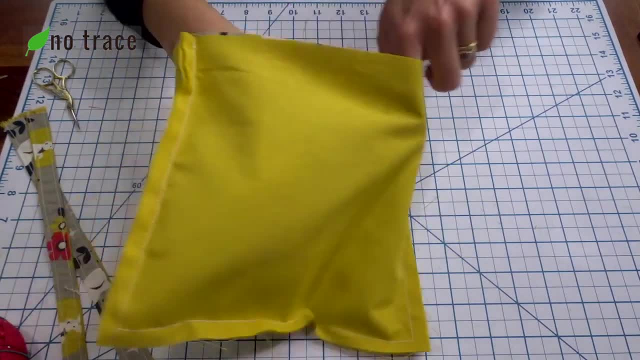 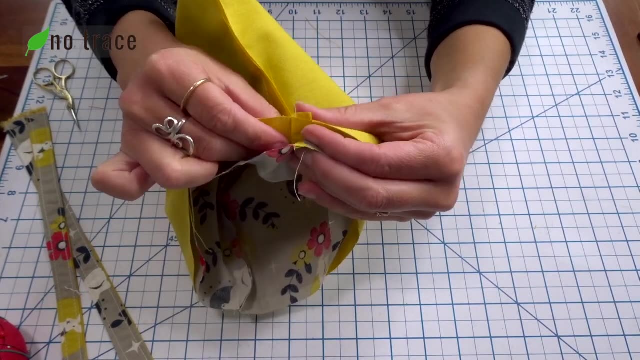 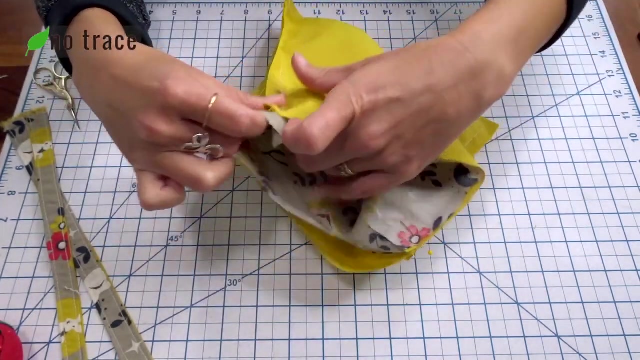 and push it down into those corners. Okay, now what you wanna do is find your side seams with the inner and the outer fabric and line them up nicely. Line them up nicely with each other and go ahead and get a pin right there to hold it in place. 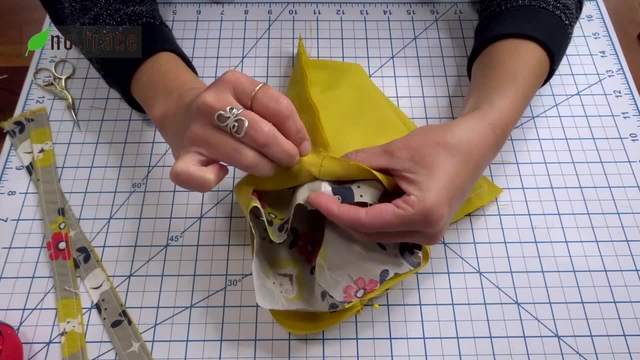 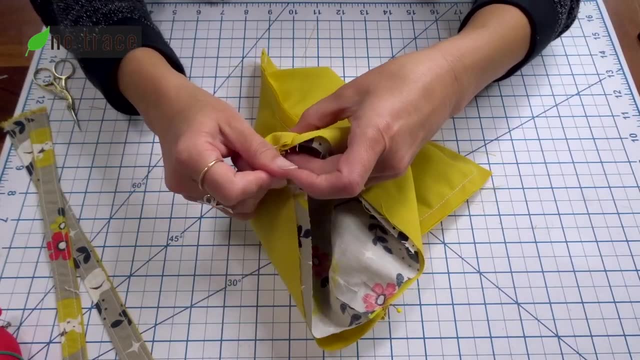 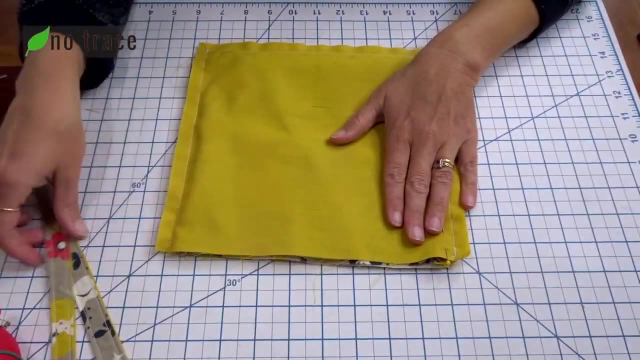 Repeat that with the other side seams: Make sure that they are aligned, and then get a pin in it And make sure, make sure, that the outer is inside there. And now we're gonna add our straps in between these layers, And what I like to do is 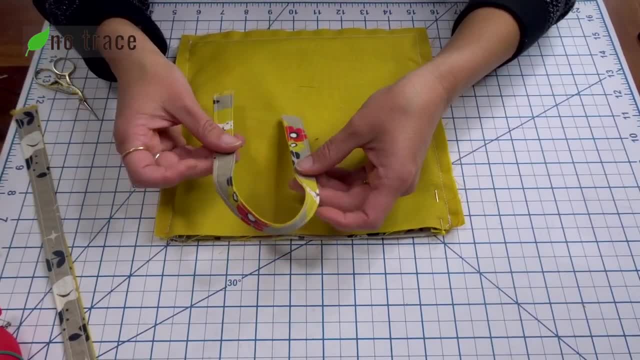 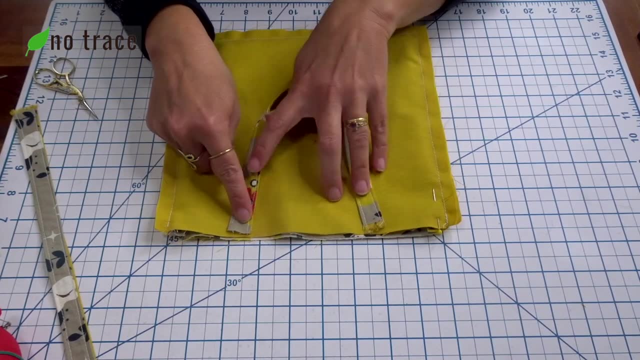 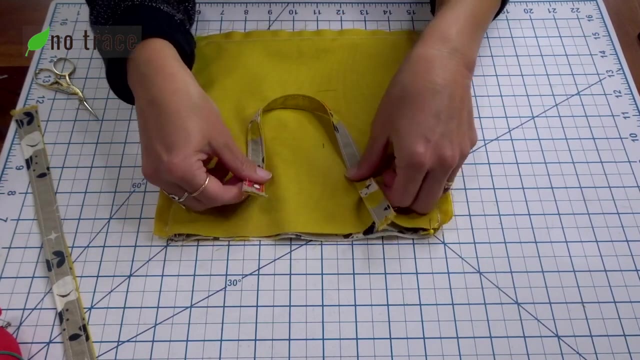 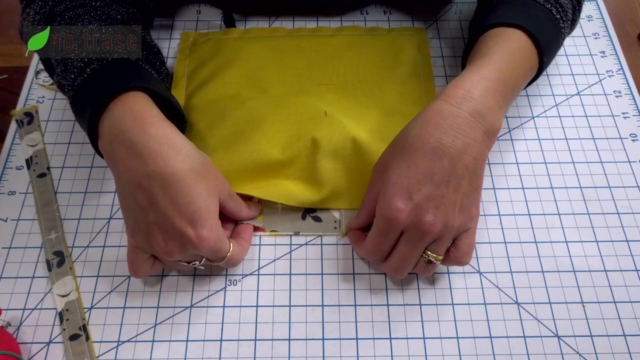 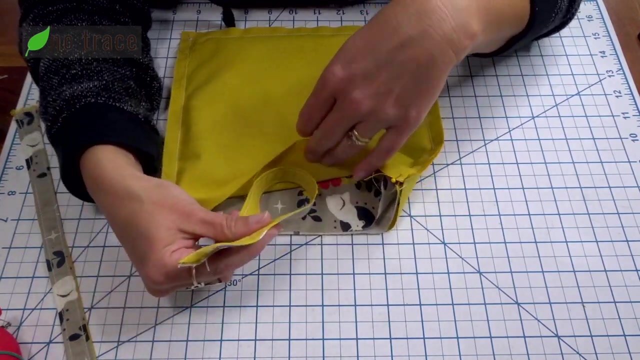 the sides and we want this to go pointed down and we want to line up the sides two inches away, line up the straps, I mean two inches away from the sides. okay, so we're putting this inside the bag between the two layers and actually I'm going to flip it this way so that the outer layer of the strap faces the outer. 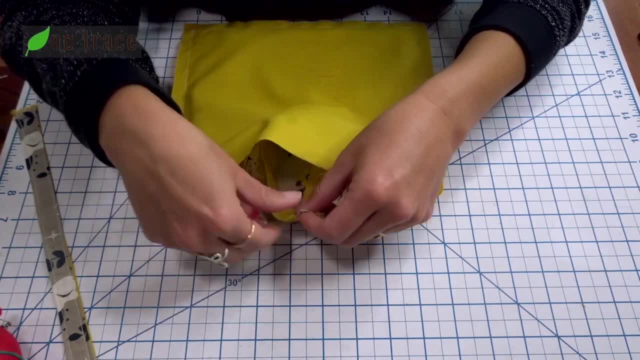 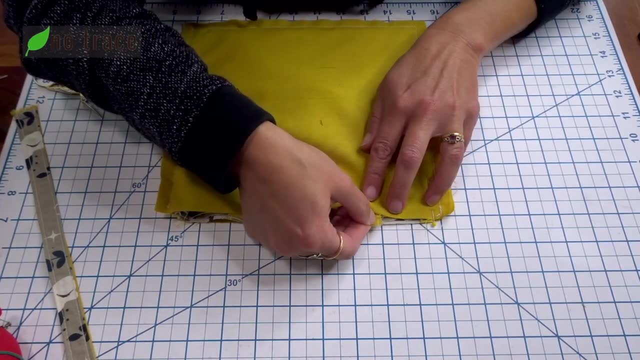 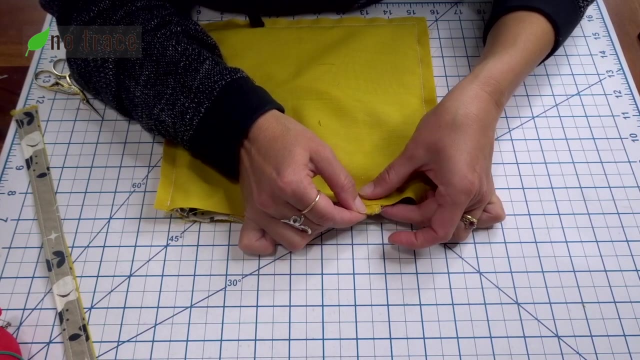 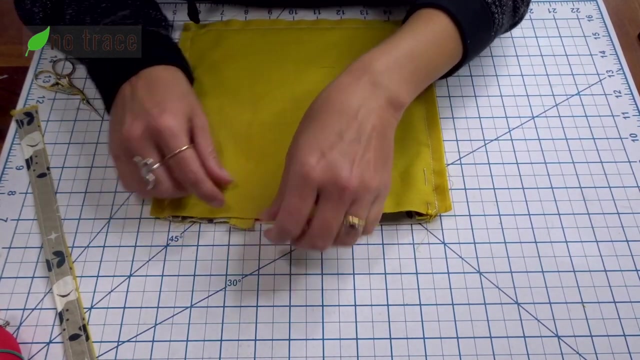 layer of the bag, get that inside. and now I want the straps to be two inches from the edges and I want my straps to stick out about a quarter to a half of an inch and get a pin in there and repeat that on this side. so this strap which you can see here is two. 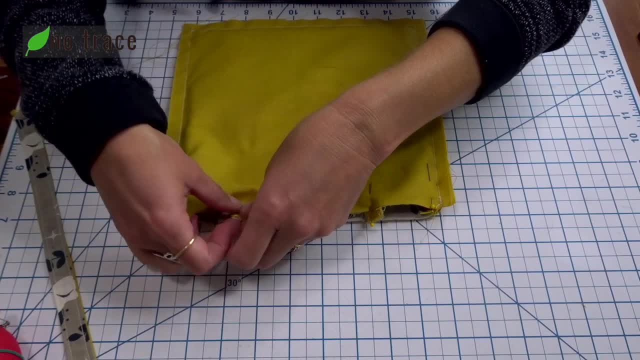 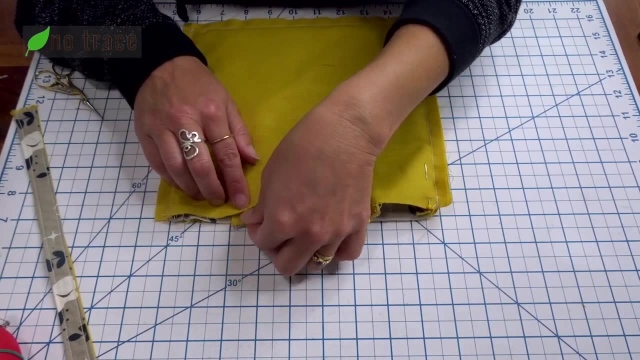 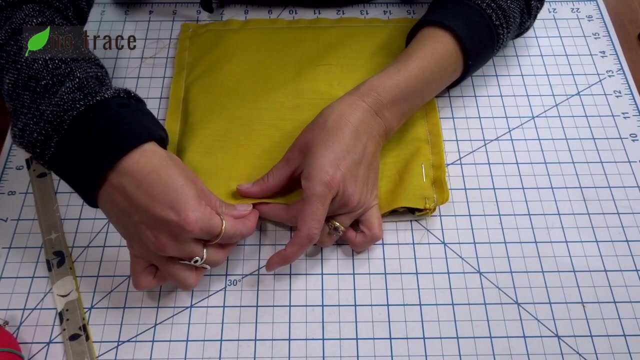 inches away from this seam. well, now it is. now it's two inches away and I have about a half of an inch of the strap sticking out. okay, and you want to try to make it as parallel to the side seam as you can so that it's not? 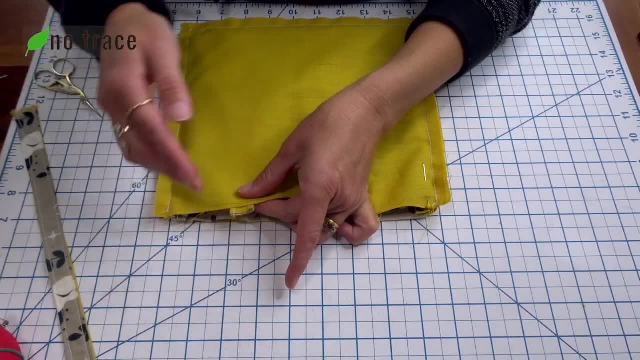 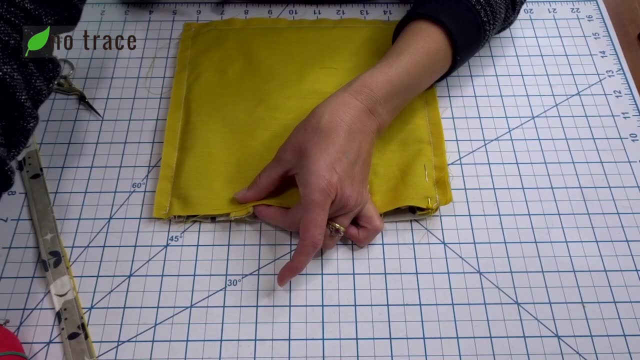 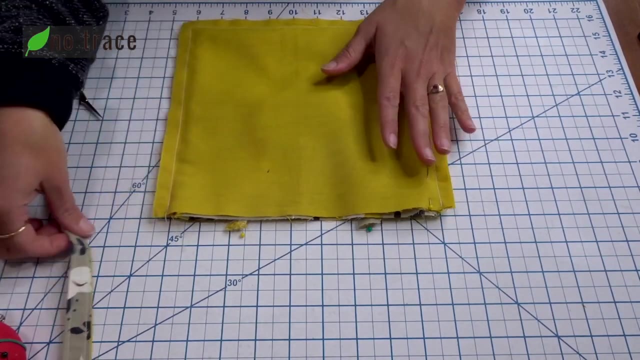 in your bag at a crooked angle. you want to try to make it nice and straight here, okay, so two inches from the edge, and then go ahead and pin it. okay, and then flip the bag over and repeat that same process. so I am placing the outer layer. 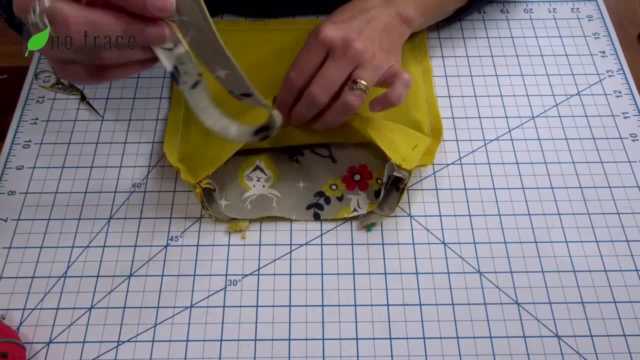 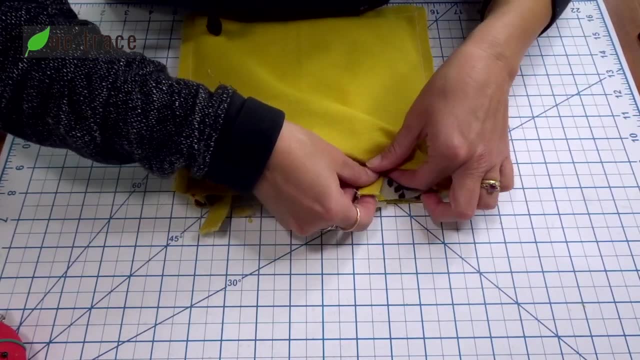 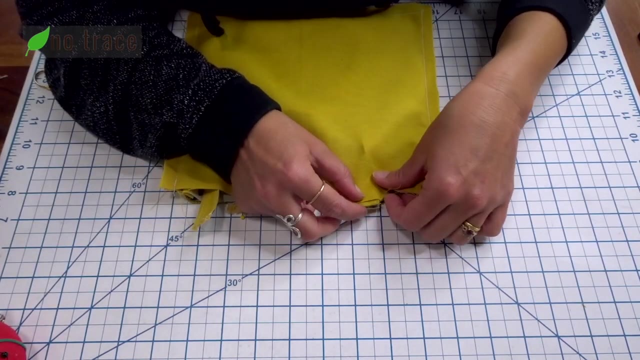 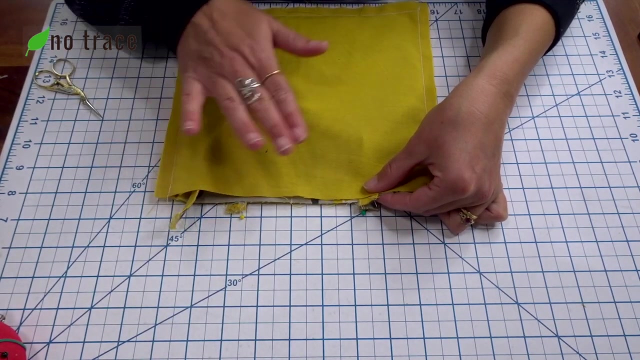 fabric so that it is touching the outer layer of this strap. and again, I'm lining up the strap with the side seam, so it's two inches from that side seam, and you can also line it up with the other strap so that when you have your bag in your hand you'll see that the straps are aligned. 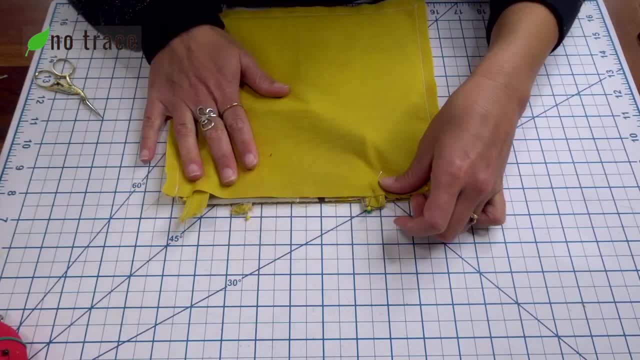 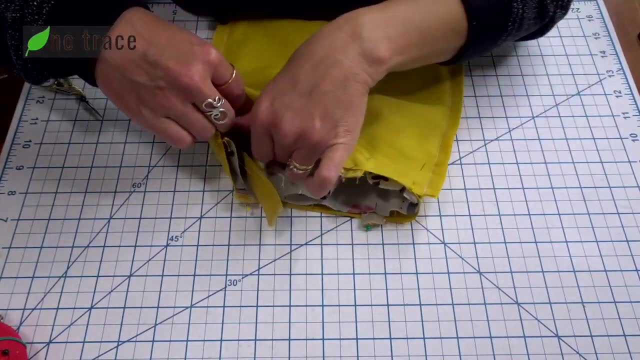 so you can use the other straps as a guidepost to double check that your strap didn't get twisted in here. you know it's kind of hard for you to see, but I can tell it's not twisted. and then I'm lining up this strap with the. 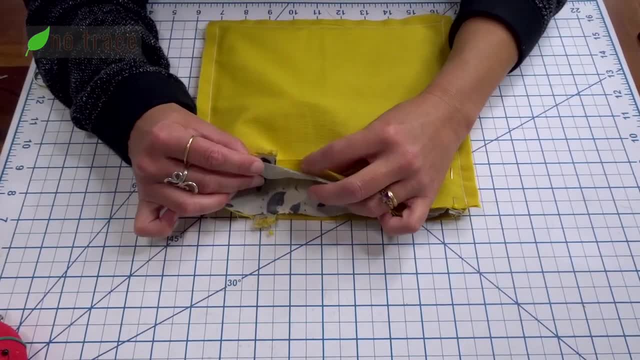 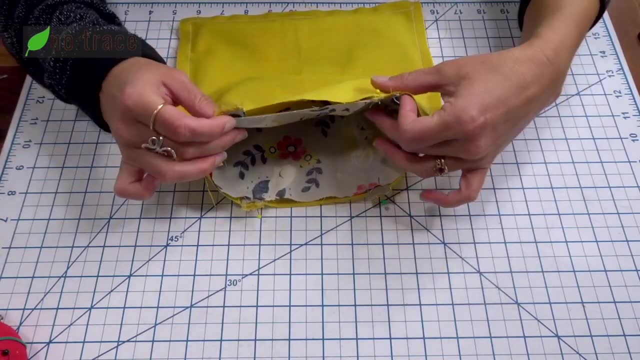 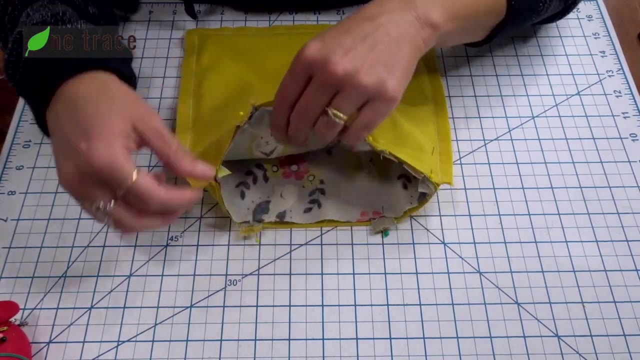 other strap and I'm pinning it just between these two layers. okay, so I still have these are not. these layers are not all connected. okay, this, this strap is between these two layers, this strap is between these two layers, and then these straps are between those two layers so that I have a bag that I can. 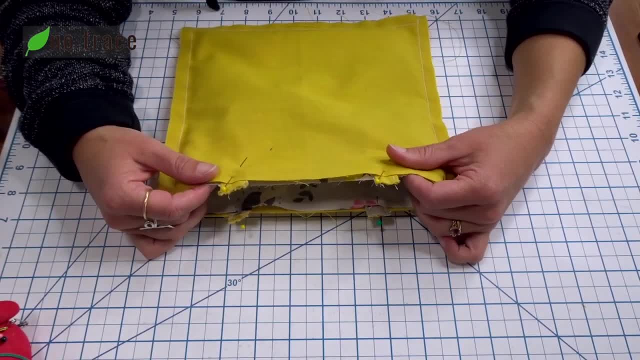 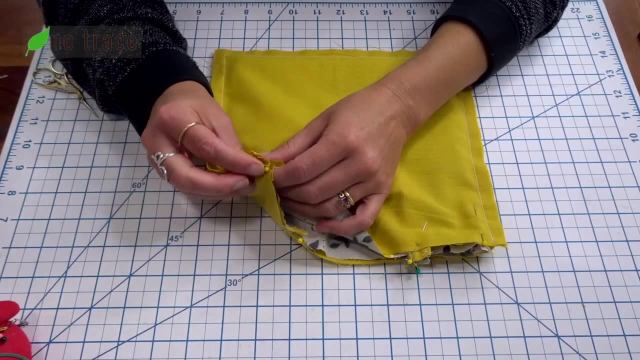 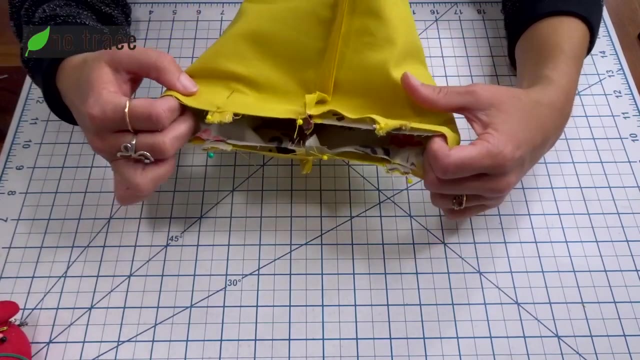 get used and actually put things inside of okay. so once the straps are pinned and they look like they're gonna be pretty well lined up, we are gonna take this to the machine and we're gonna stitch all the way around this top edge with a half inch seam allowance. we're gonna leave an opening on this side, so we're not gonna. 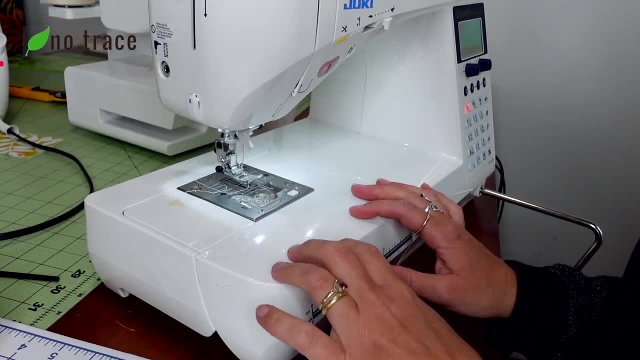 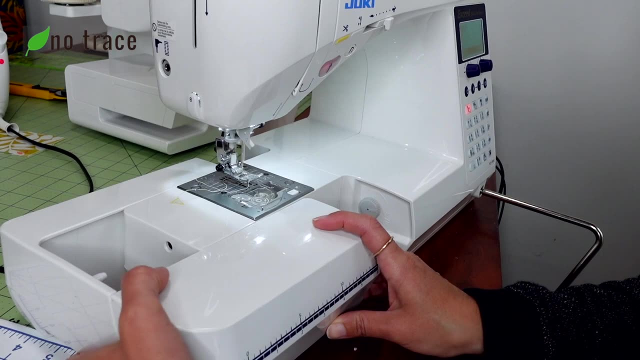 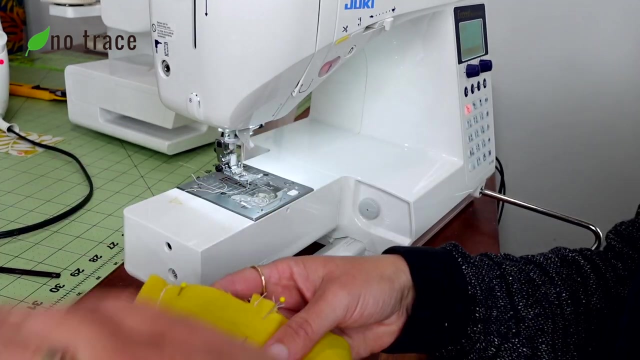 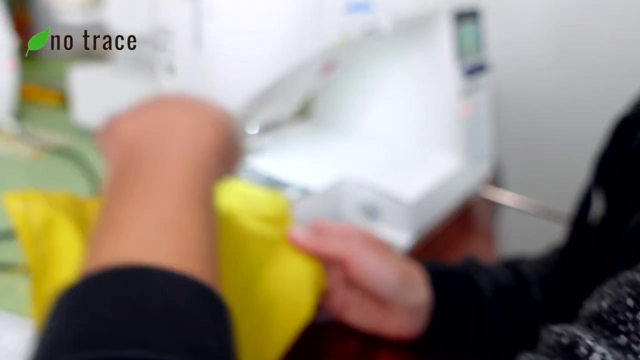 stitch this area closed back at the machine. you might find it helpful to take this, this large sort of carriage part, off your machine and set it aside so that you can just sew around this part of your machine. and we're gonna start right just before this strap. it doesn't matter which strap just start, right before one. 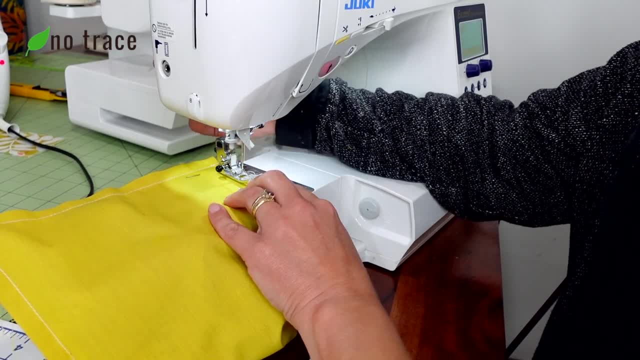 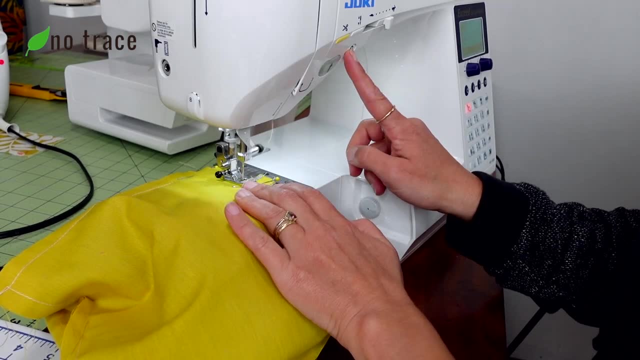 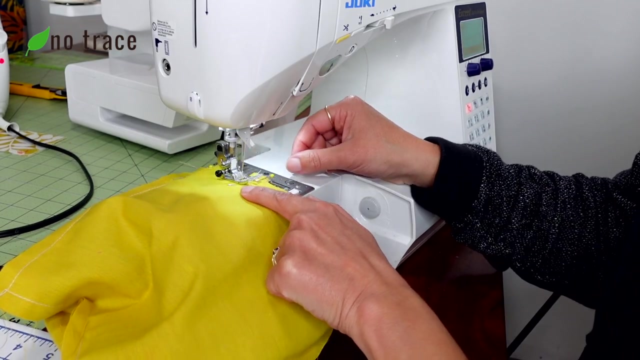 of the straps. we're gonna do a half inch seam allowance. make sure to do a back stitch at the beginning. oops, a little back stitch, and then, as we sew over the strap, we're gonna reinforce it. so we're gonna go over it. take that pin out and 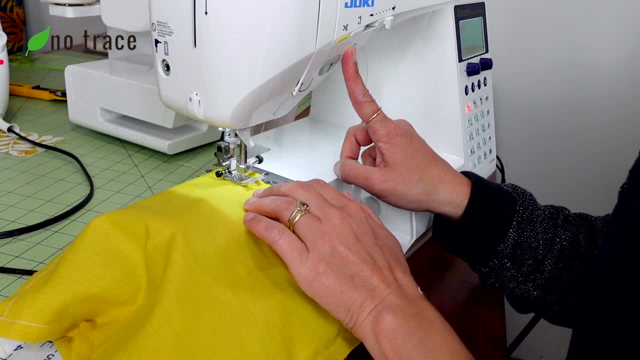 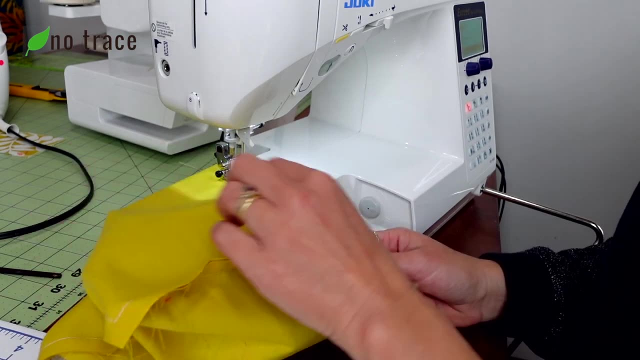 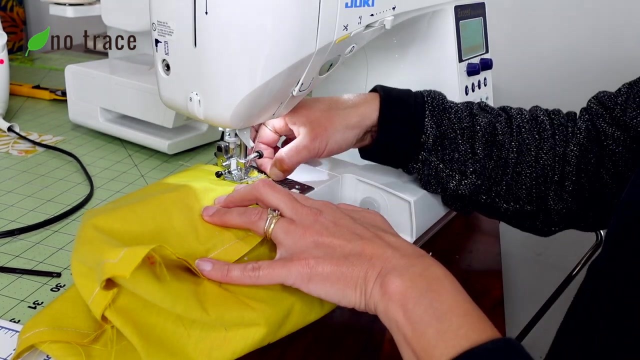 then go back so reverse, stitch over it again and then go over it once more, and then, when we get to this strap, we're gonna do the same thing. so we're gonna pick our pin out, so all of the straps are pinned together. we're gonna make sure to stitch all the way around. 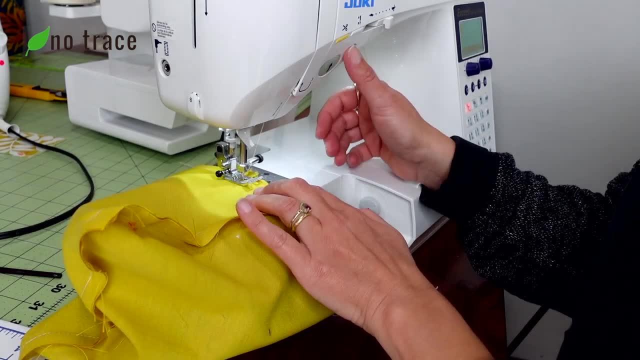 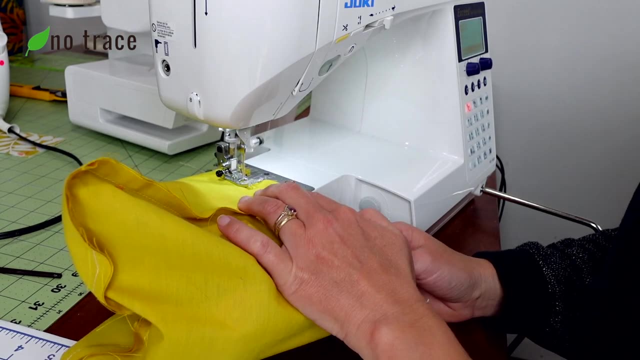 okay, and then when we get to this strap, We're gonna do the same thing. so we're gonna take our pin out, so all the way along, all the way over the strap, and then reverse And repeat that on the remaining straps. All right, we're at the last strap. 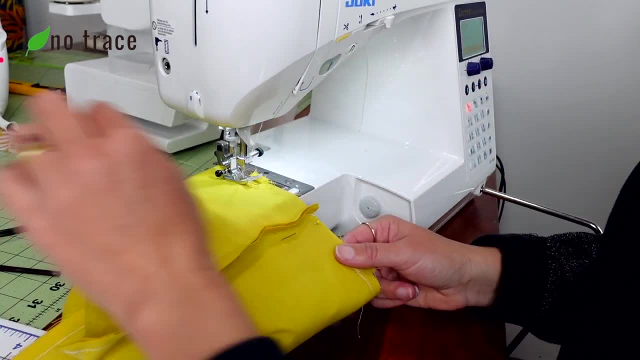 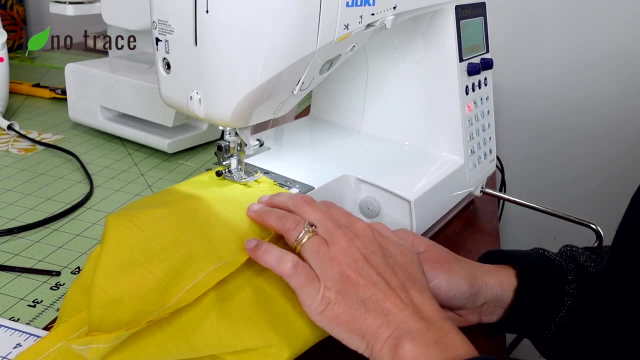 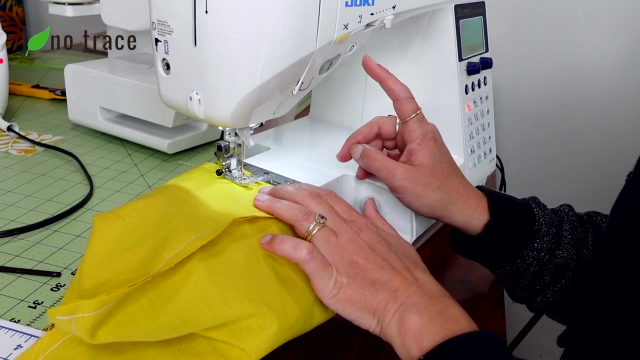 so we're gonna go take that pin out, we'll go over it and then reverse and then go over it a little more and then just go slightly off the strap and then back stitch and stop so that we have an opening to turn our bag right side out. 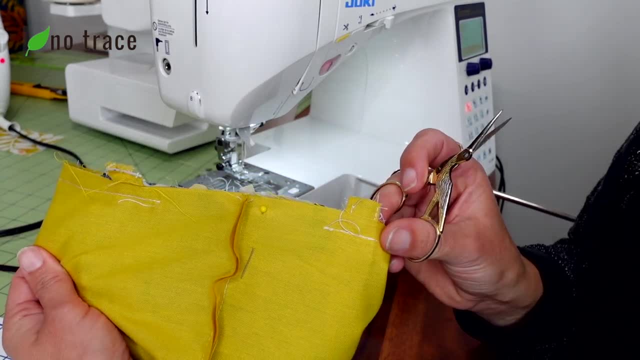 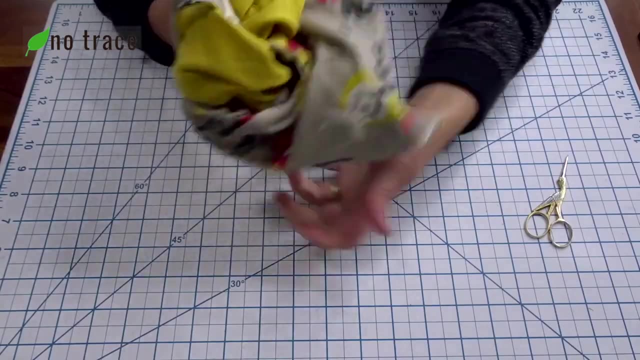 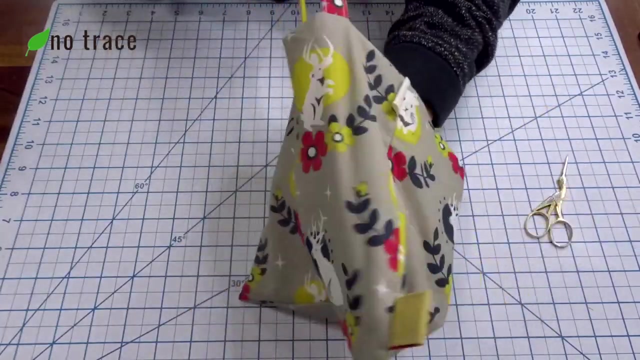 So we still have this opening to turn our bag around. So go ahead and take the pin out and then use the opening to turn the whole bag right side out and get that lining into the bag. Oh my goodness, it's so cute. 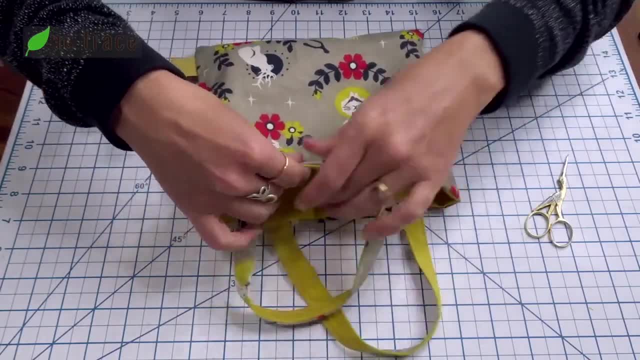 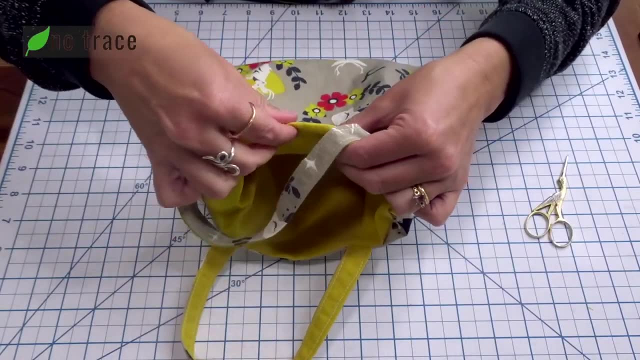 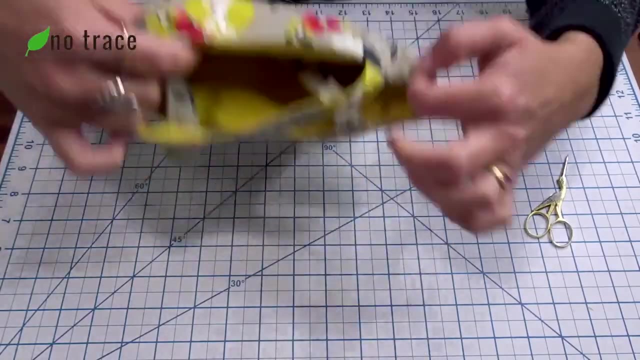 And use your fingers to roll out the seam along the top edge, except for the open spot. But we want this area to be as flat as possible, And then we're almost done with our adorable mini tote. So we're gonna go ahead and iron this. 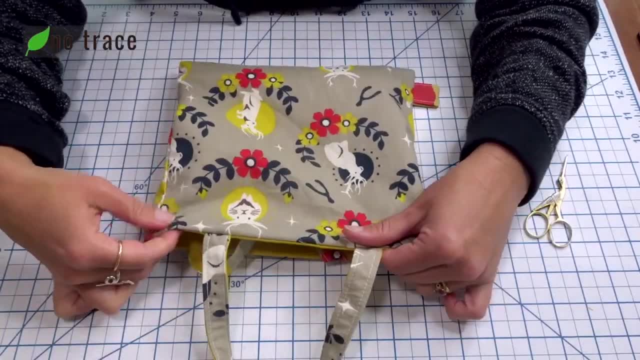 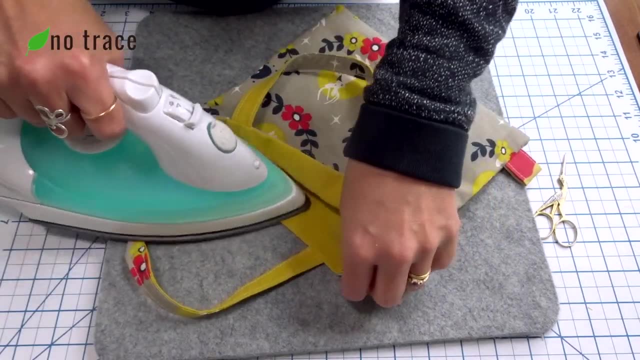 flat iron. this top seam flat all the way around the bag. Now if you have an ironing board, this might be a little bit easier, but you can also just do it on a flat ironing mat like this one. Just get the iron in there. 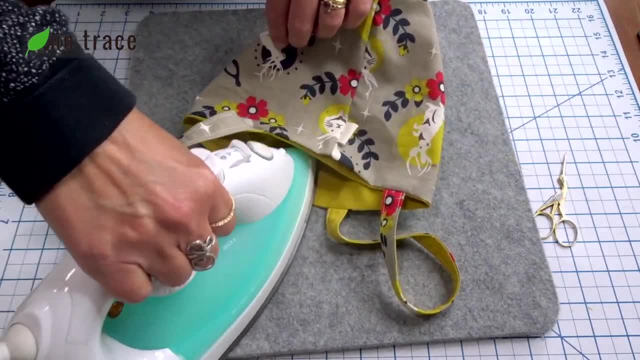 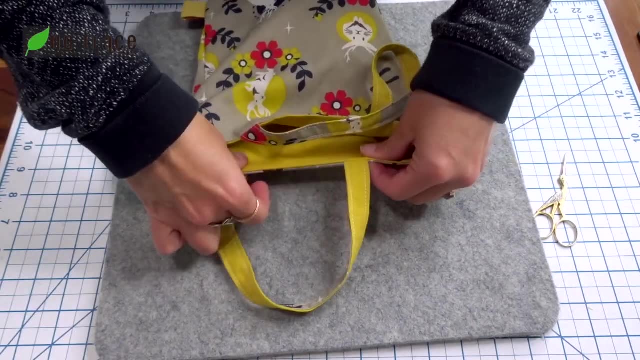 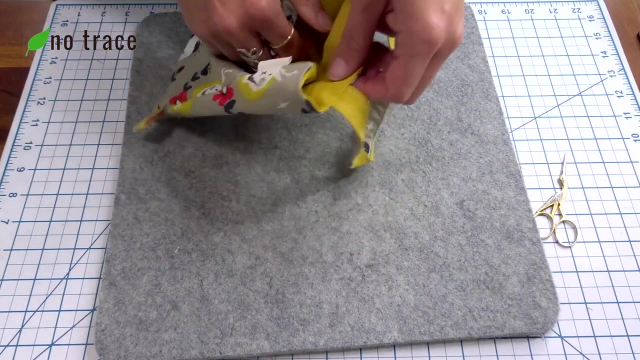 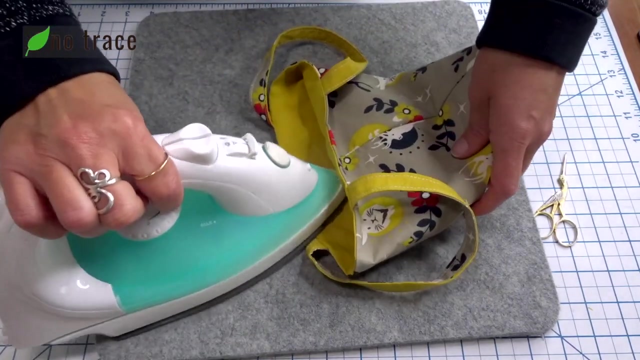 and reposition the bag as you need to. And as you're turning the bag, you wanna also double check that your seam is in place. Seam is still laying pretty flat And get this spot as well. Okay, now we're ready to sew. 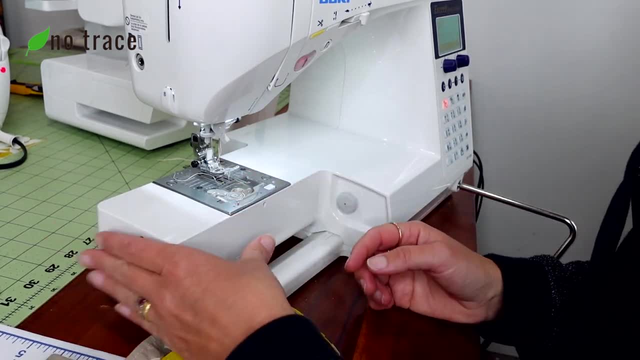 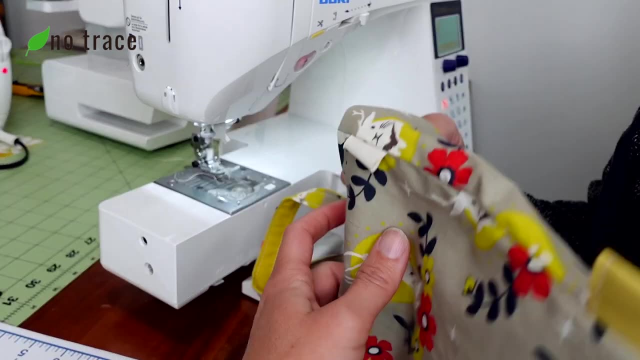 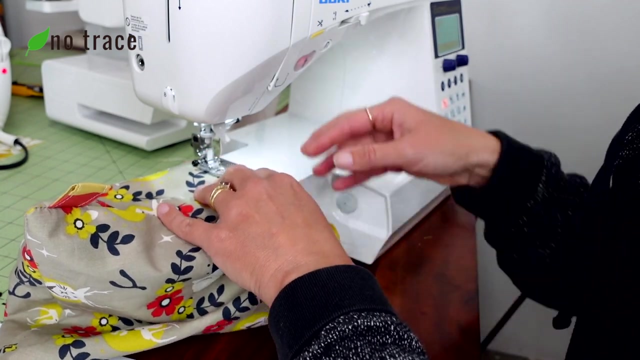 Okay, back at the machine. I still have the big storage drawer off, the little shelf off, And I wanna start at the opening here over on the side. So go ahead and get this open area under your presser foot And we're gonna go all the way around. 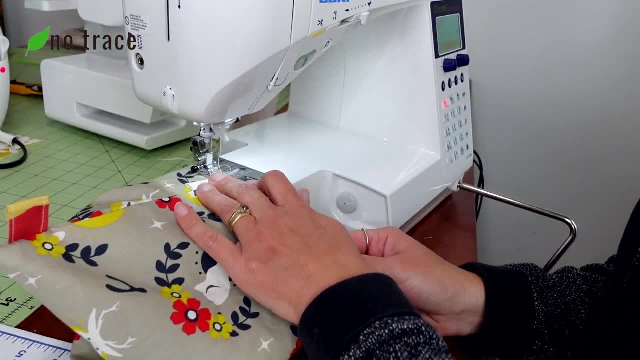 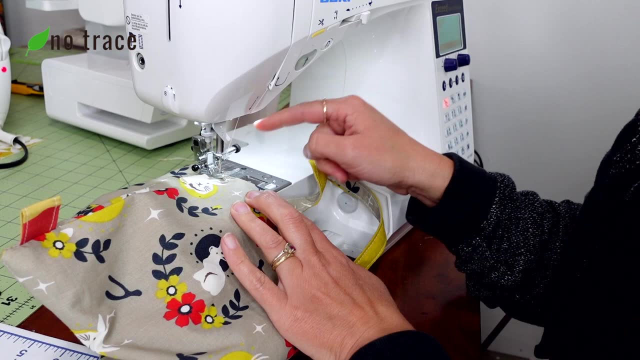 with a 1 1⁄8 inch seam allowance, So real close to the edge. Now I'm not doing a back stitch when I start, because I'm gonna come back around to my starting point at the end And that's when I'll do a back stitch. 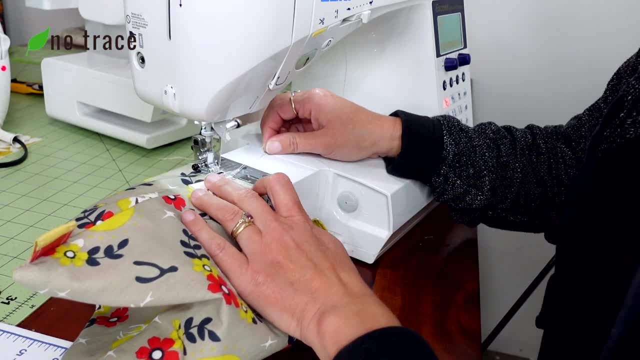 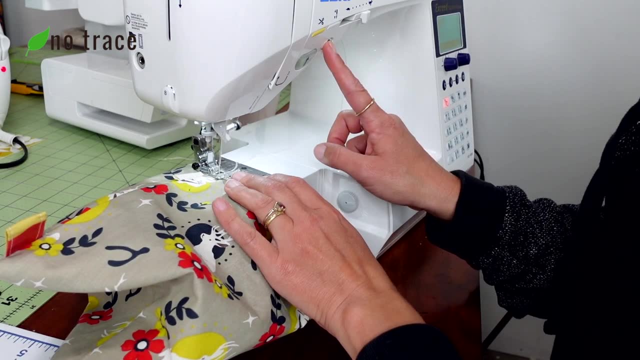 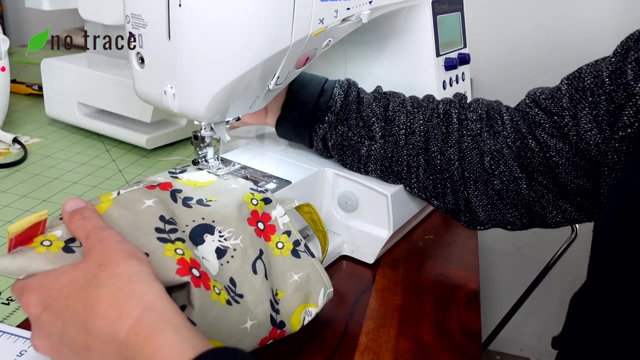 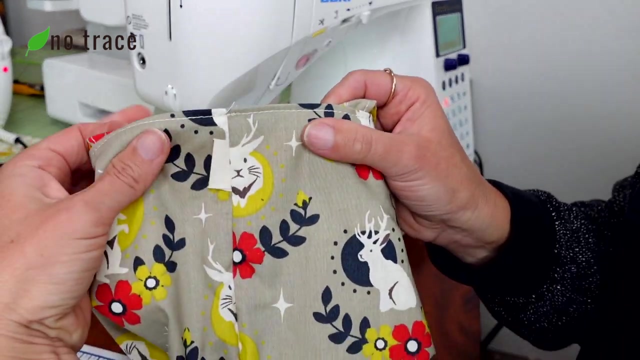 So I'm back at my starting point. So I just wanna go over my original stitches a few times with a few stitches, and then reverse, and then go over them once more. just a few stitches and then we're done. So your final spot should look like that. 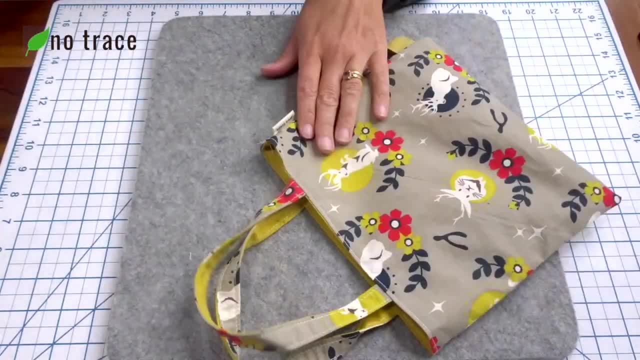 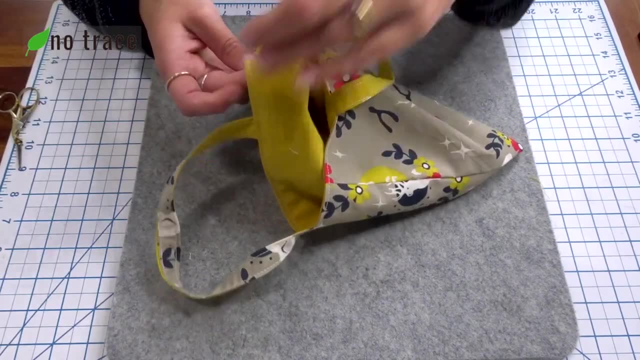 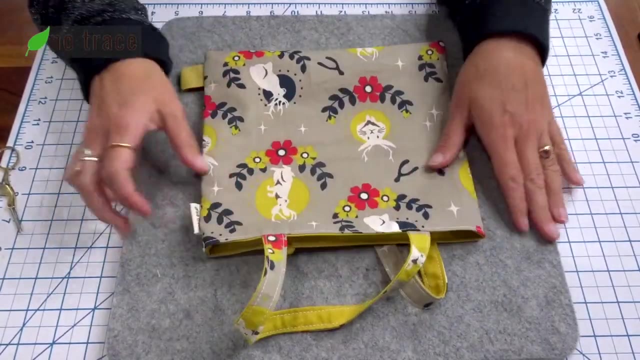 All right, So the next steps are to check the bag for any loose threads. So I'm gonna trim these from my last row of stitches, And there's a couple here. I don't see any other loose threads, which is kind of surprising. 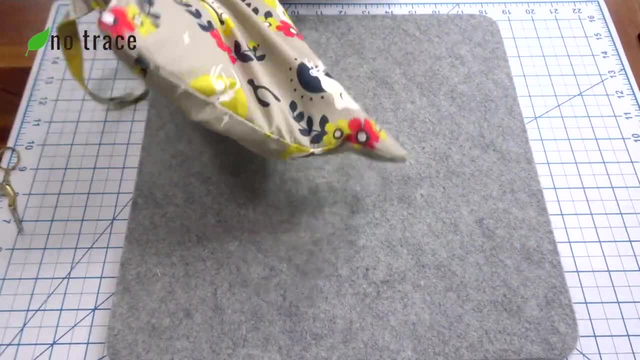 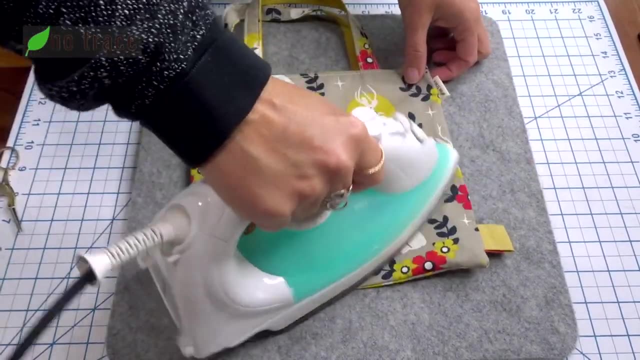 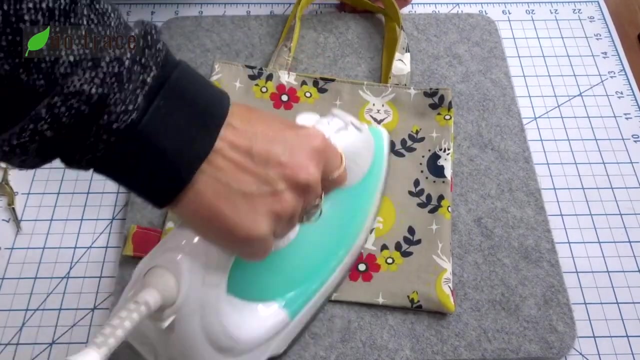 And the last thing I'm gonna do is I'm gonna give it just a little press so that it lays nice and flat, So just like that. Oh my goodness, it's so cute. I think my daughters might fight over this bag a little bit. 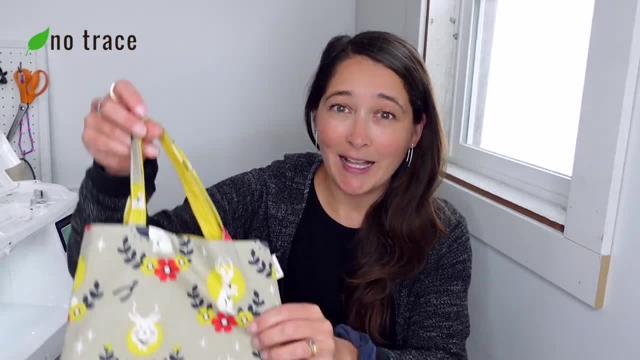 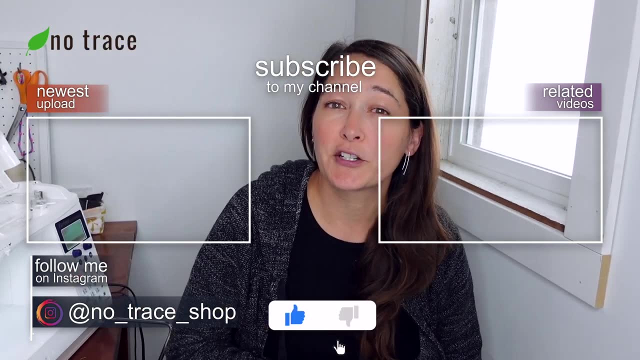 Thanks so much for watching this video. I hope you get out there and make some cute little totes for the little ones in your life. Please give this video a thumbs up and subscribe to the No Trace channel to get notified about all of our videos. 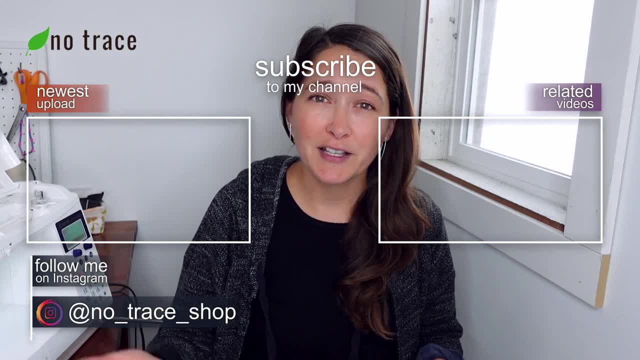 We put out a video every single week on zero waste, sewing and crafting and living tips. So I'll see you again very soon.